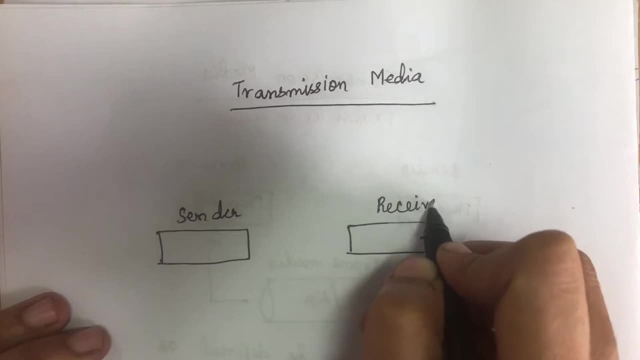 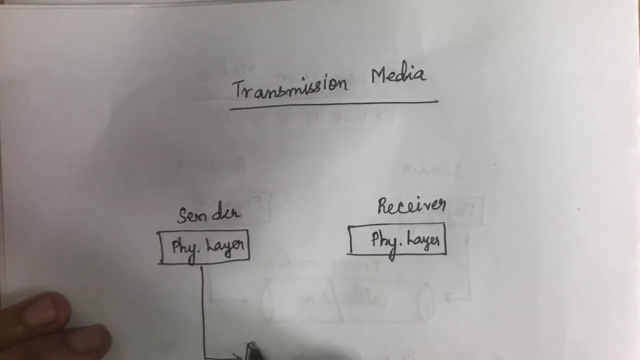 and this is the physical layer, and this is the physical layer of the receiver. When a message has to be transmitted from the sender to receiver, it has to be from the physical layer, it has to be sent to the transmission media. Through the transmission media, the message will 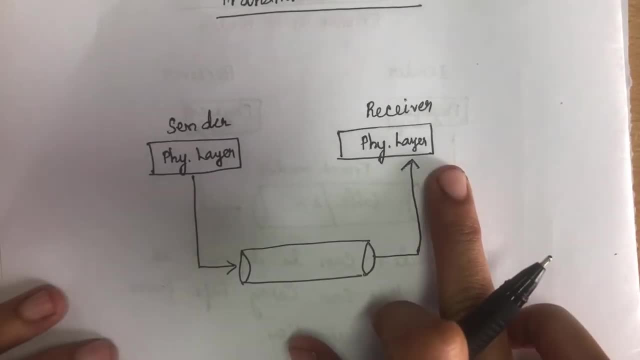 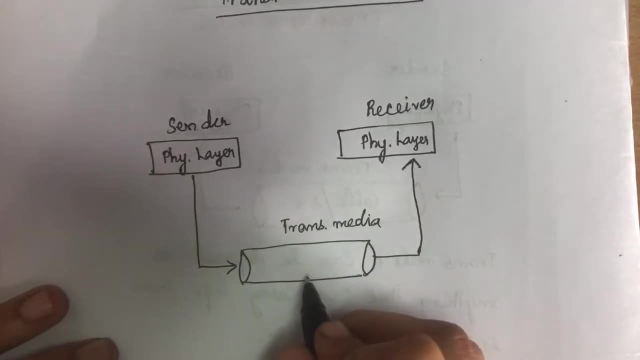 be sent and it will be given to the physical layer on the receiver side. So this is the transmission media. This transmission media, it can be wired or it can be wireless. If it is a wired one, we will be using a cable, and if it is a wireless one, we will be transmitting through air. Okay, so we can. 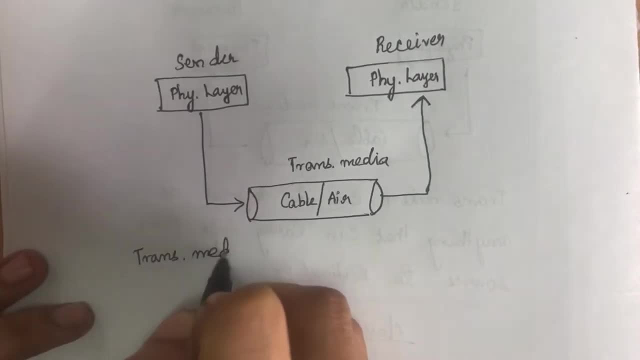 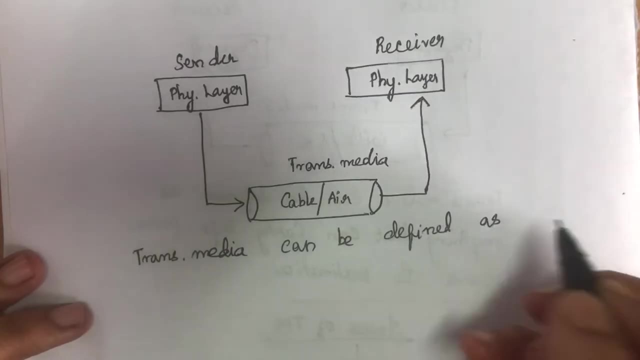 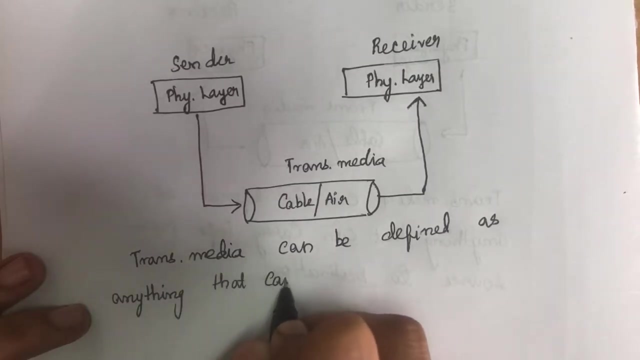 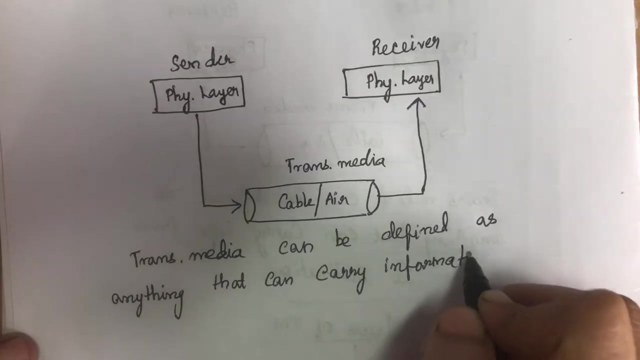 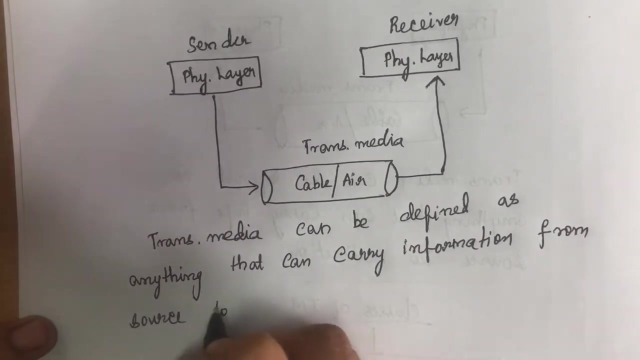 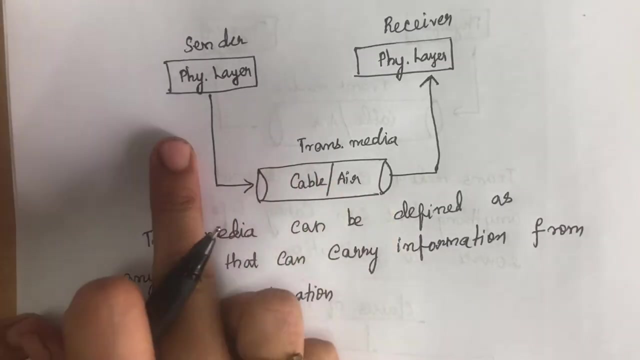 define the transmission media as transmission media can be defined as anything that can carry information from source to destination. destination is called as transmission media, So it can be a media which carries information from source to destination, that is called transmission media. Next we will see the classes. 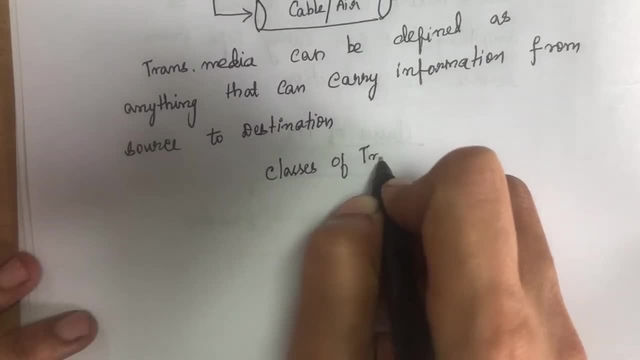 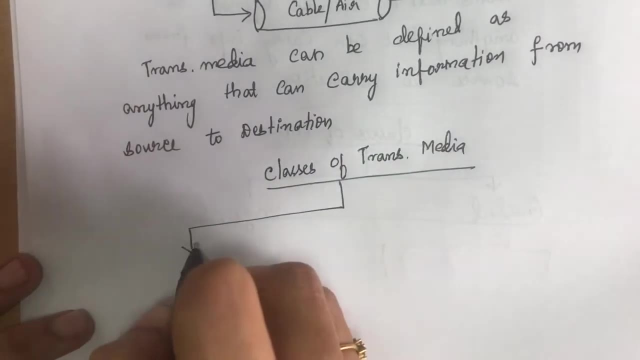 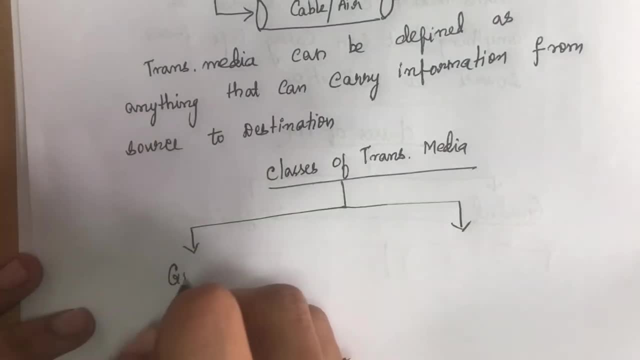 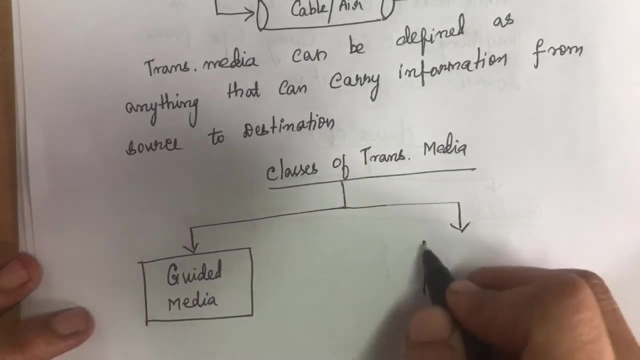 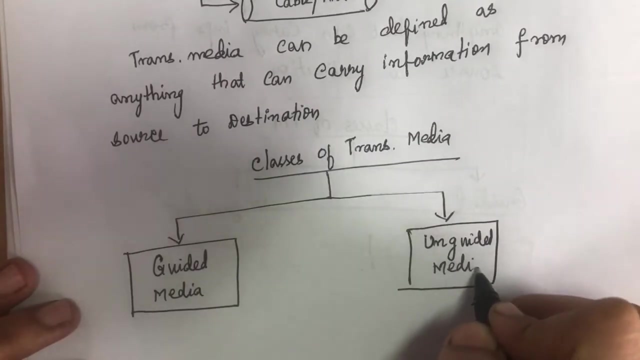 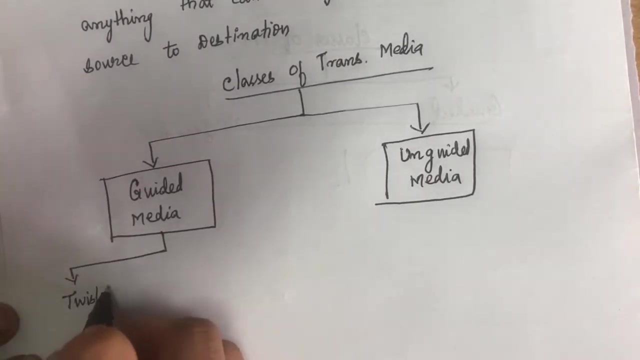 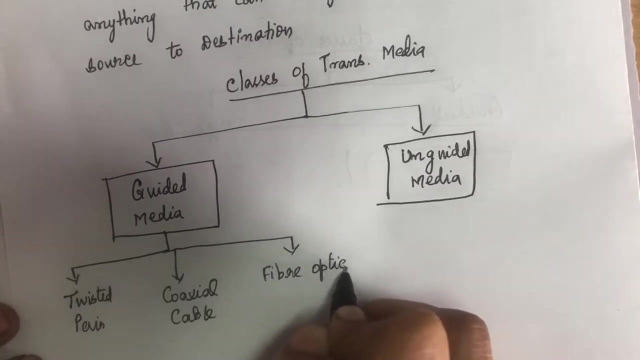 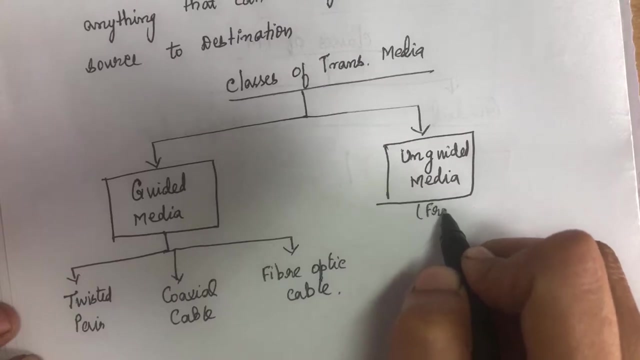 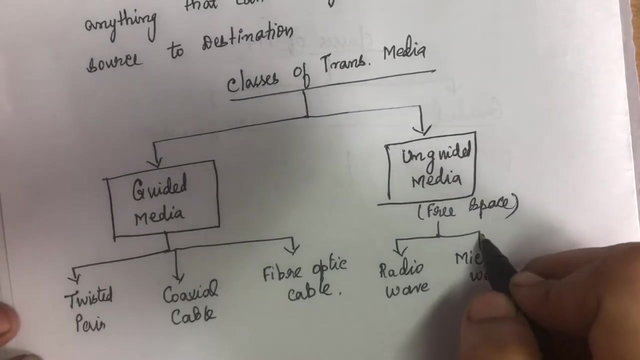 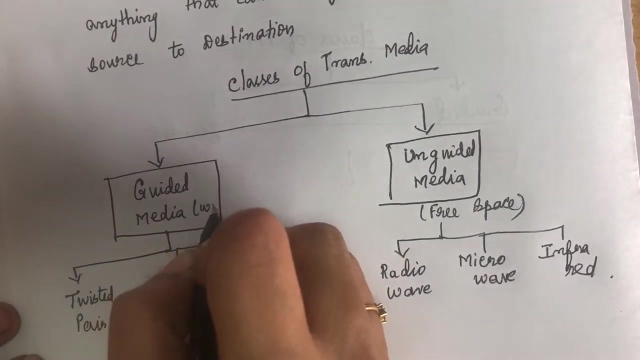 RAT, he fried and done this. salon chef media is ID and again classified into a focusedations, brekya and fiber optic cable, so unguided media. it is a free space okay. so this is classified into radio wave, microwave and infrared wave. so this guided media is a wired one and unguided. 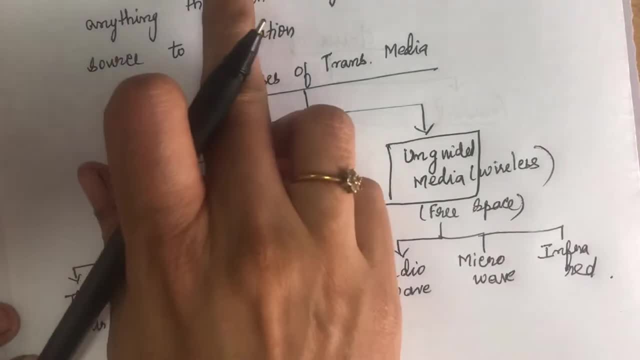 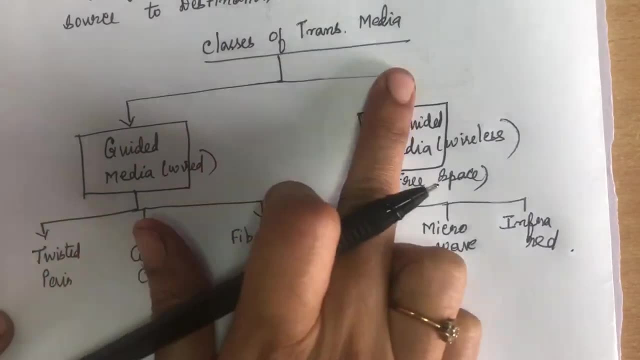 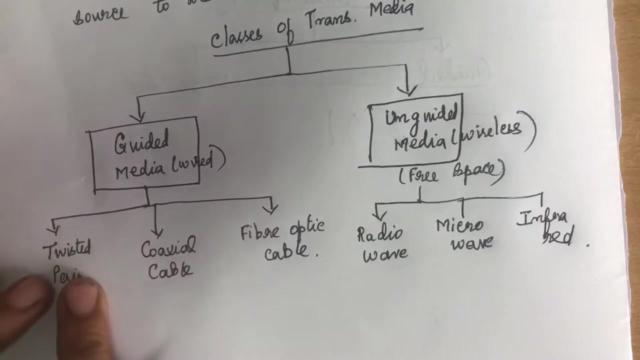 media is the wireless media. so here when we are transmitting the signal, it will be transmitted through the cable. so when it is transmitted, the types of transmission media are guided one and unguided one. in the guided media it is wired one, it is again. 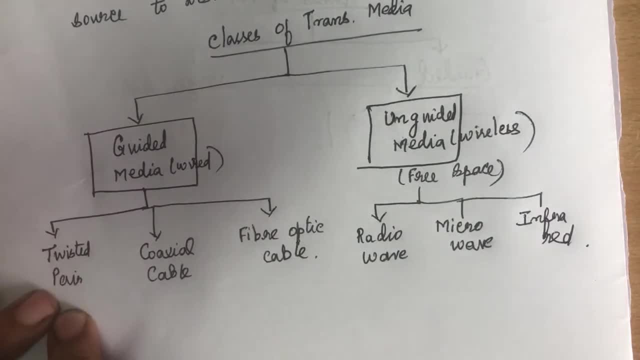 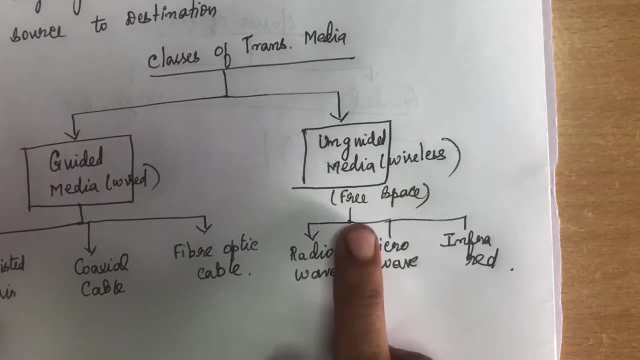 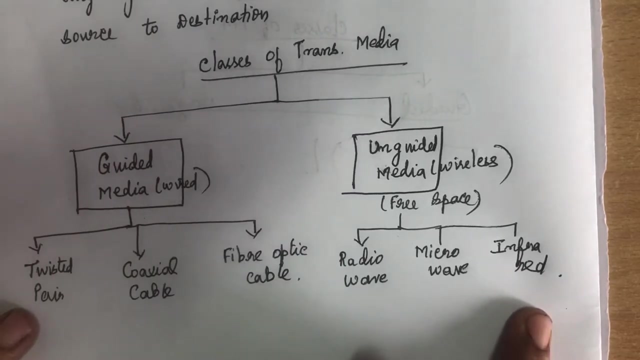 classified into. we can use a twisted pair to send them information, or we can use coaxial cable, or we can use fiber optic cable. coming to unguided media, it is, it will be transmitted through free space, so we will be. we can use radio wave, microwave or infrared wave. 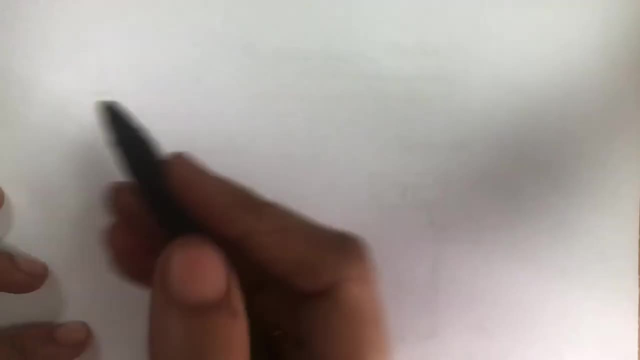 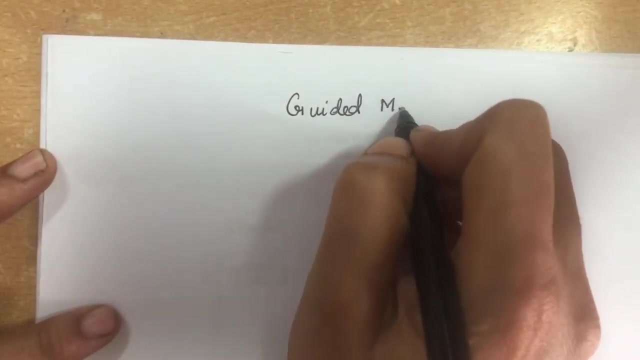 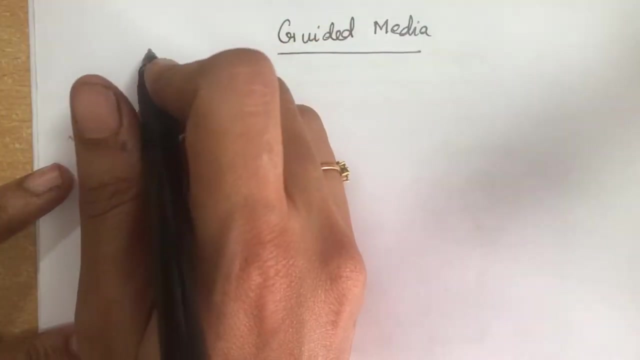 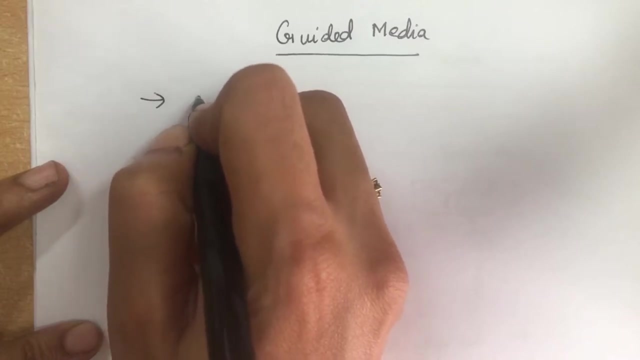 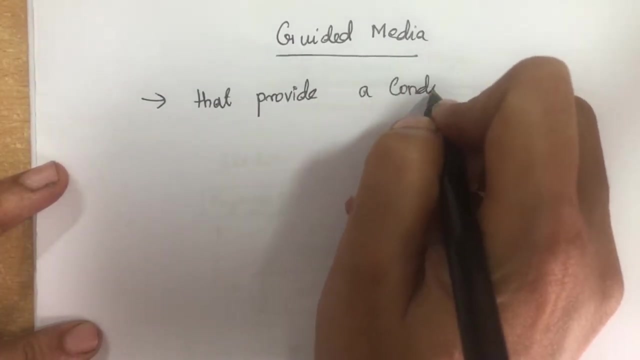 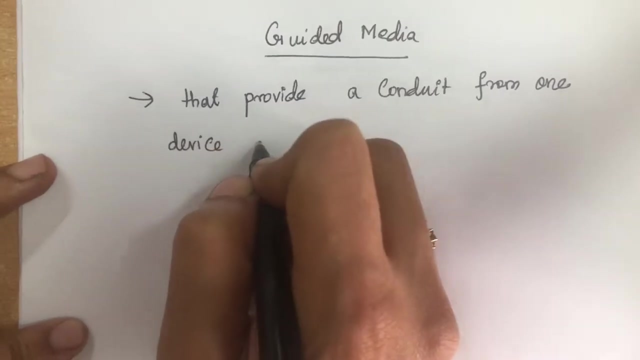 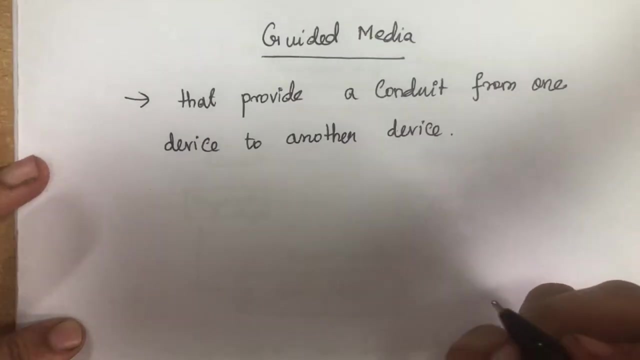 for transmission. Now we will see in detail about guided media. so guided media, it is. or those that provide contact from one device to another device. so guided media, or those that provide a contact- okay, Okay, Okay, Okay- From one device to another device through a cable. so it is broadly classified into. 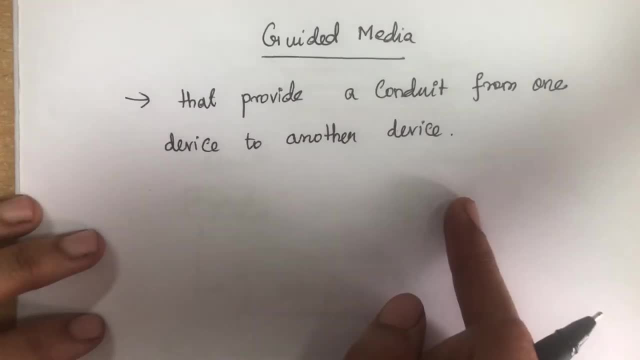 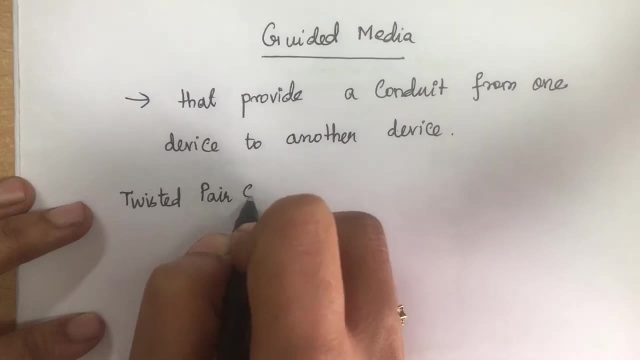 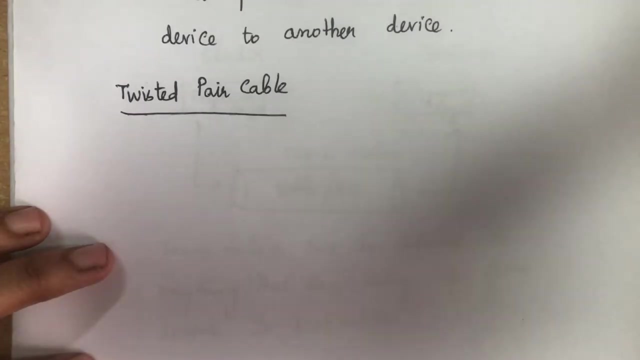 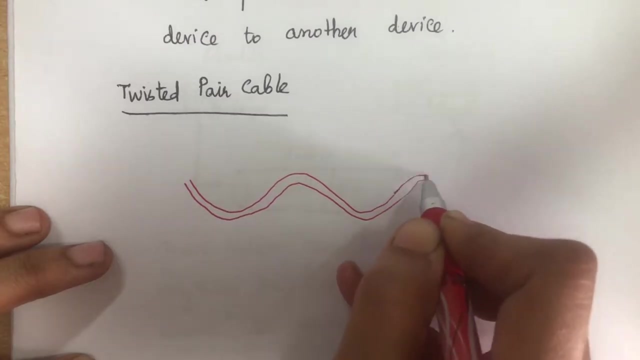 twisted pair cable, coaxial cable and fiber optic cable. So first we will see in detail about twisted pair cable. Coming to twisted part cable, it is. it consists of two insulated copper wires, So it is arranged in a spiral pattern. So this is one wire. 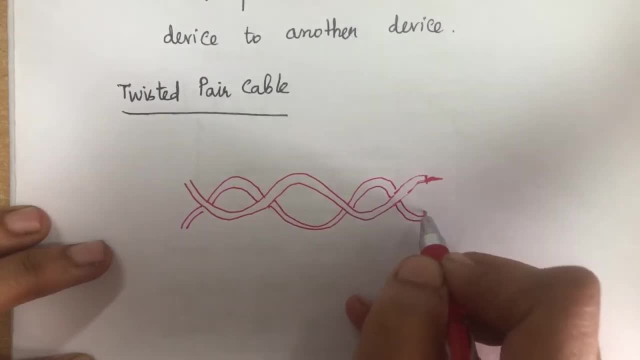 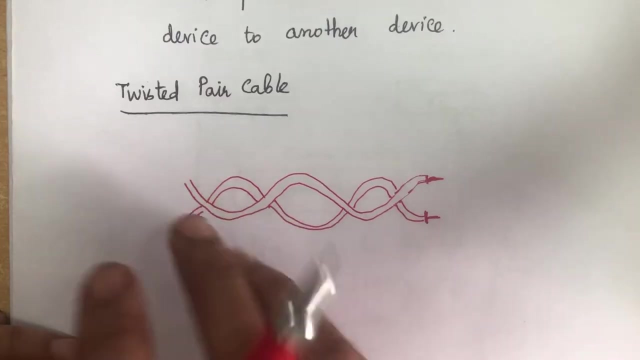 One more wire. So this is your twisted part cable. it consists of two insulated. it is made up of copper wires. It is arranged in a spiral pattern and twisted together. So this is the twisted part cable. So here, one of the cable will send the signal. 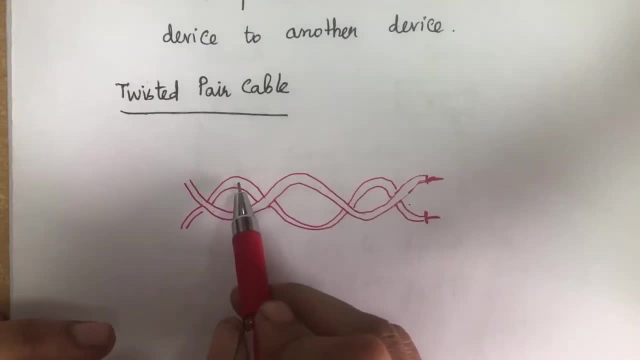 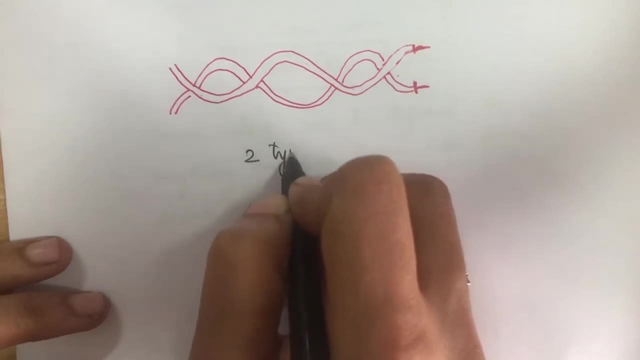 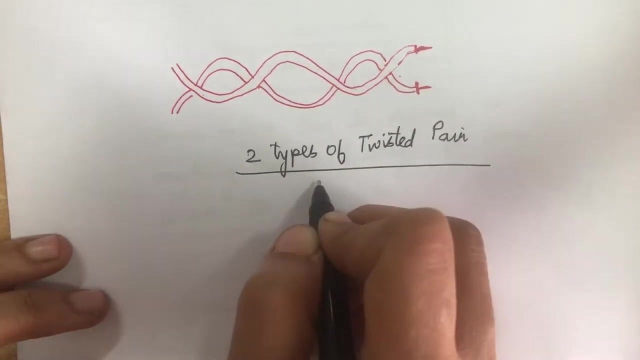 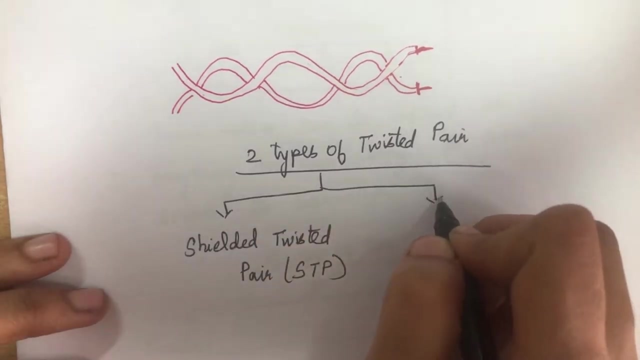 One of the wire will send the signal and other wire will act as the ground reference. So there are two types of twisted part cable. One is Shielded twisted part, or, in short, we can write STP. Other one is unshielded twisted part, in short, we can write UTP. 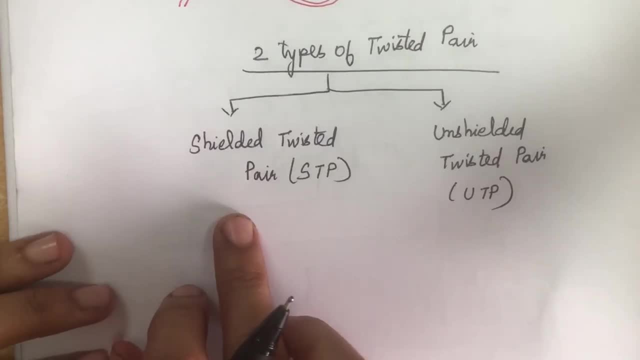 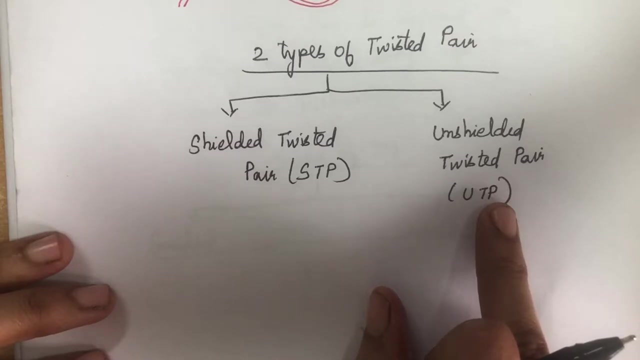 So in coming to shielded twisted part, there will be a cover to protect the twisted part. So IBM has introduced this twisted part cable and by the name itself you can say it will have a cover to shield the copper wires. But coming to unshielded twisted part, there here we will not be having any cover to protect. 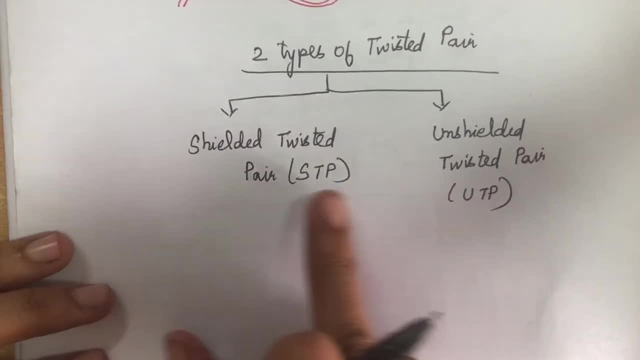 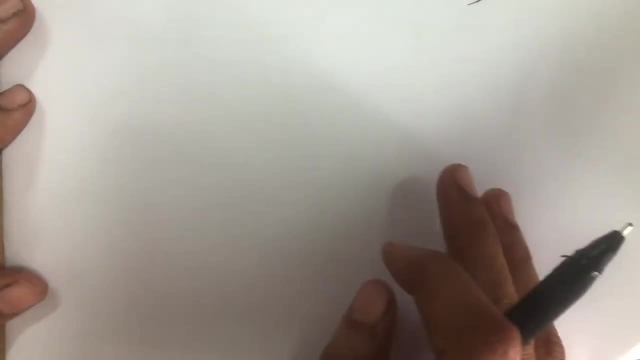 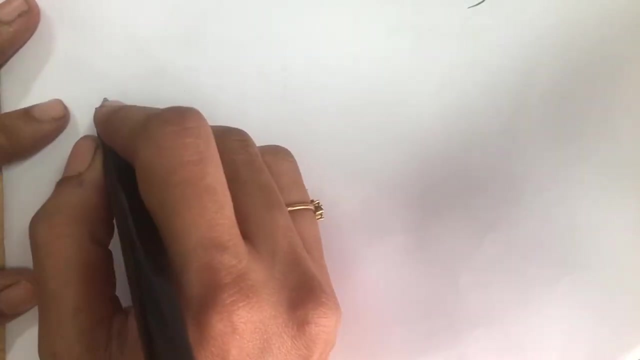 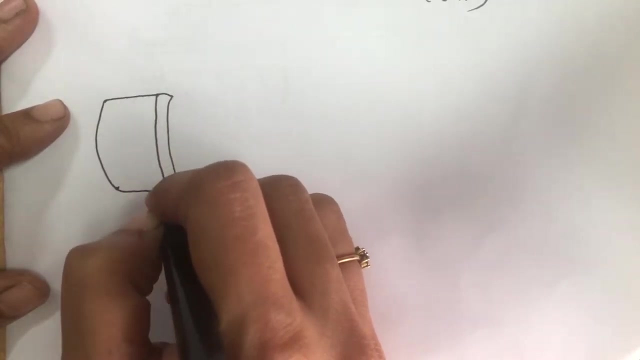 the cables. So this is all about your shielded twisted part and unshielded twisted part. Now we will see the difference between unshielded twisted part cable and shielded twisted part cable. So, coming to unshielded twisted part cable, so here there will be a plastic cover. 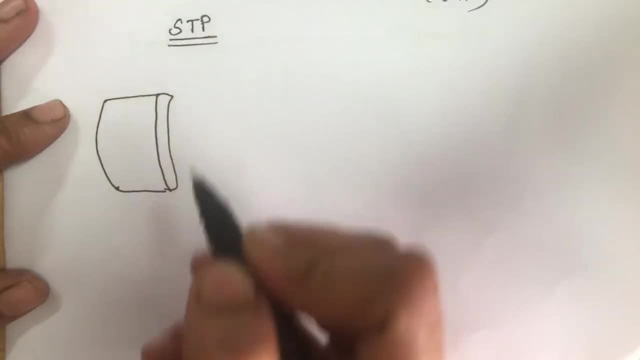 Ok, so this is shielded twisted part cable and after which you have a metal shield, or you can say that it is a braided mesh. It is a mesh. So from here, This is shielded twisted part. This is shielded twisted part. 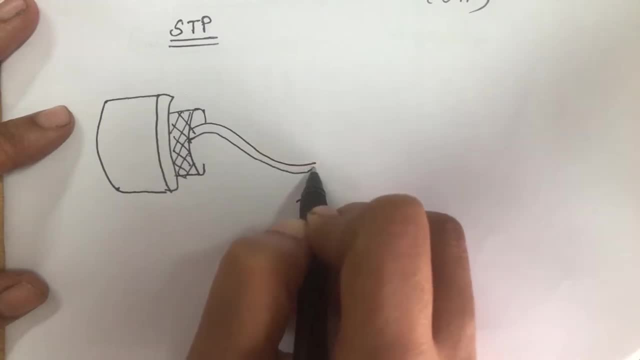 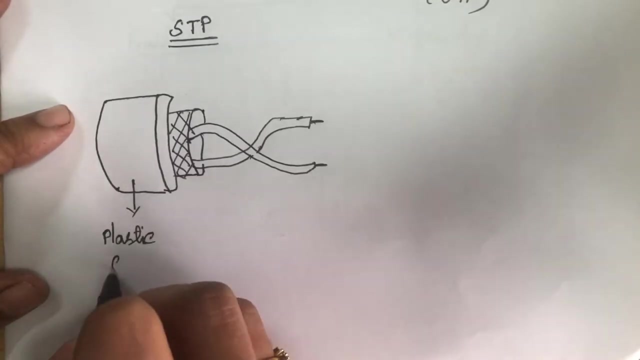 This is shielded twisted part. Here it will protect over insulated copper wire. with wire, insulated copper wire will be there. So this is plastic cover and this is the metal shield. So in shielded twisted part cable there will be a metal shield which is covering this copper understood. 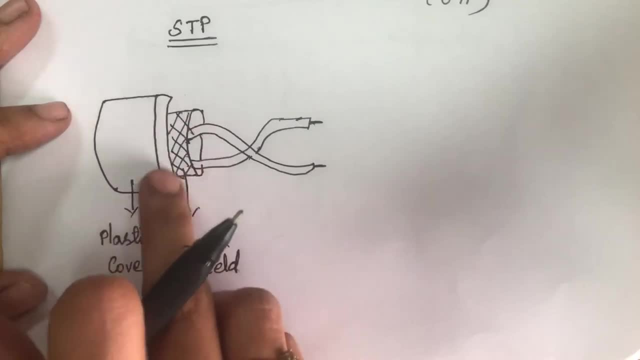 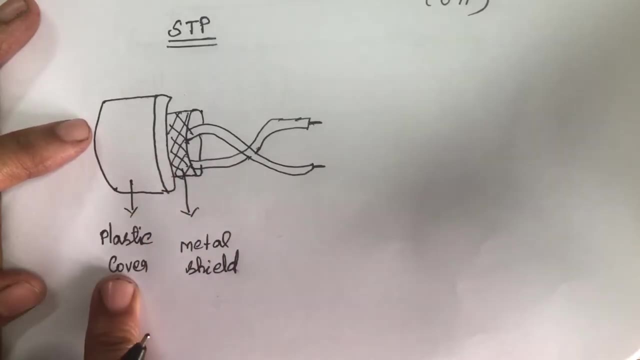 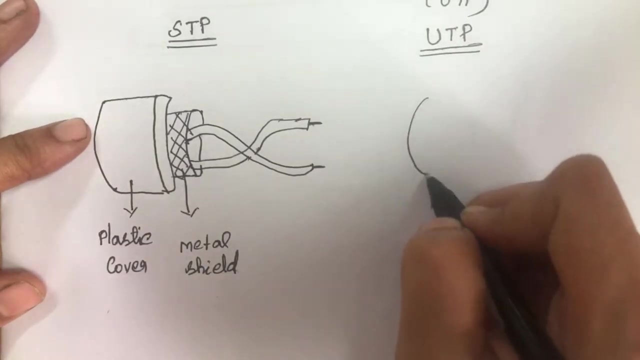 covering this copper wire. so this mesh shield will be braided and it will be in mesh format, and after which it is encased by a plastic cover. this is a shielded twisted pair cable. coming to unshielded twisted pair cable, there will be a plastic cover and after which you 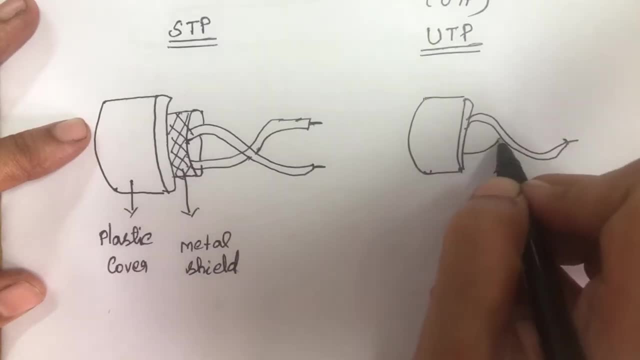 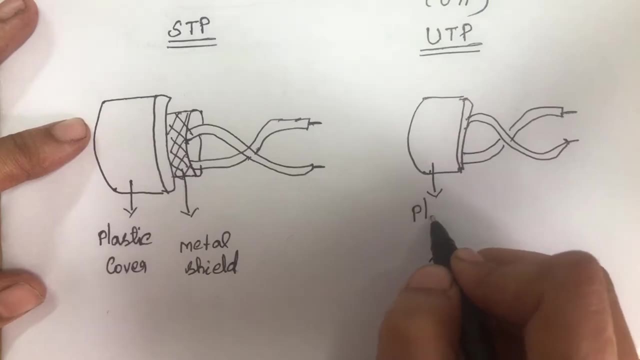 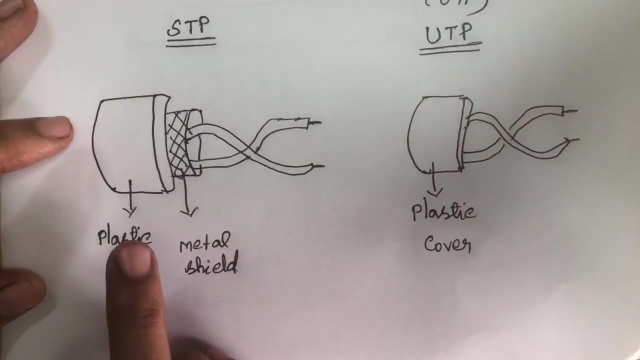 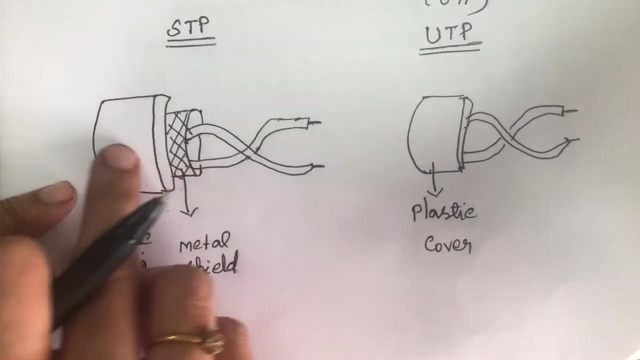 have your insulated wires, so there is no shield for covering your insulated wires. so this is your unshielded twisted pair cable. so in coming to this shielded twisted pair cable, because of this metal shield it will prevent the noise that is, or cross talk that occurs. 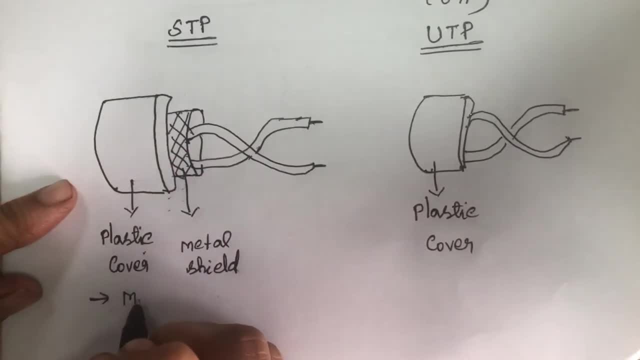 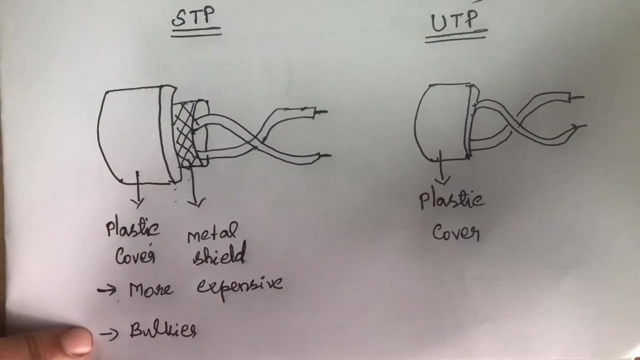 inside the cable and it is more expensive and bulkier. also, when we compare this utp cable with this stp cable, it is more expensive and it is the cable looks bulkier. this is all about your stp and utp. now we will see. 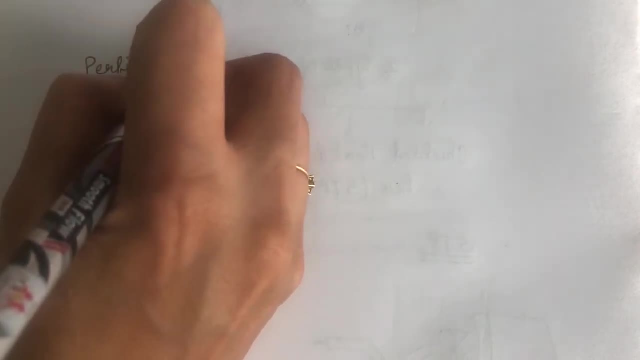 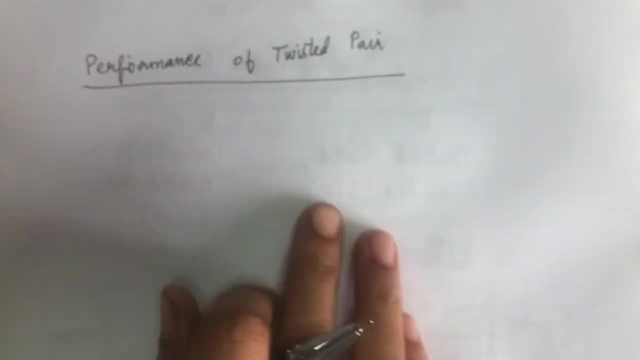 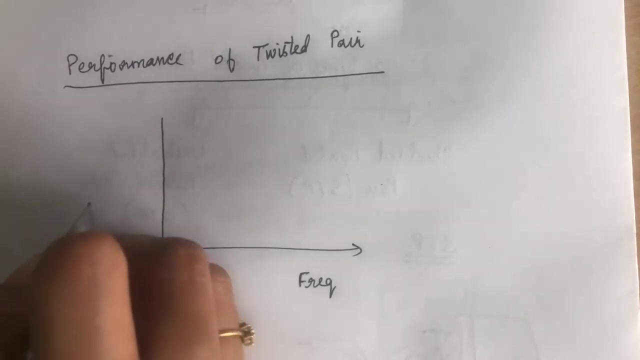 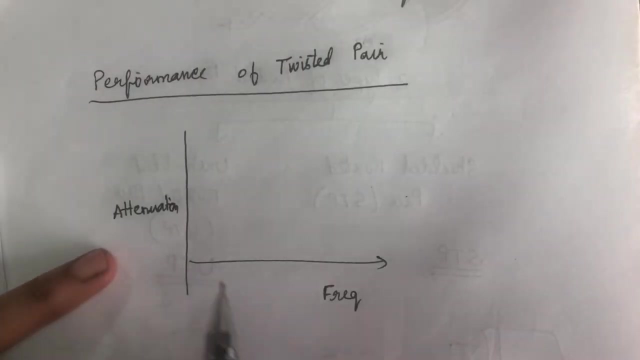 the performance of twisted pair. so coming to the performance of twisted pair. so here we are going to compare the frequency with attenuation now in this performance. so we are going to compare the frequency with attenuation. so attenuation is the loss of energy occurs when a signal is passed through the transmission medium. so it is measured in decibel. 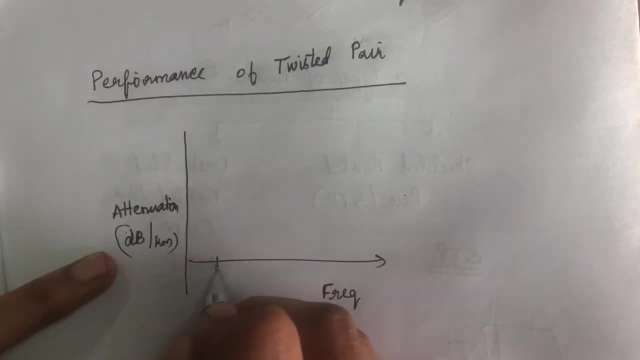 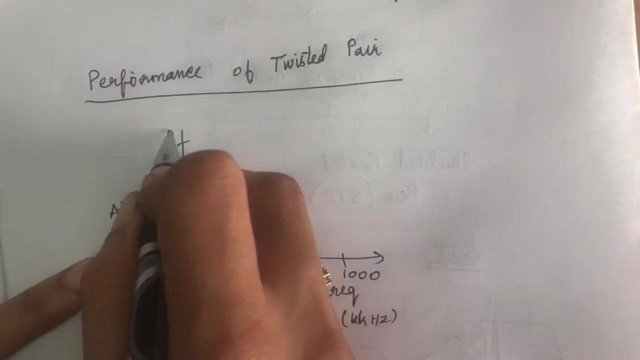 meter, by decibel, by kilometer, and this is in kilohertz. frequency is measured in kilohertz, so it is ten hundred kilohertz and thousand kilohertz. so when it is, this is attenuation- will be two, four, six, eight. so here this is what the the curve, we will get. 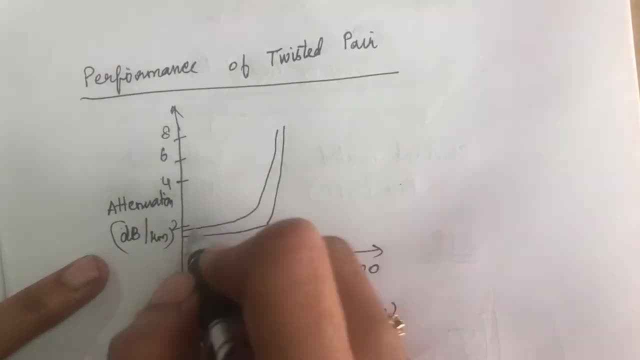 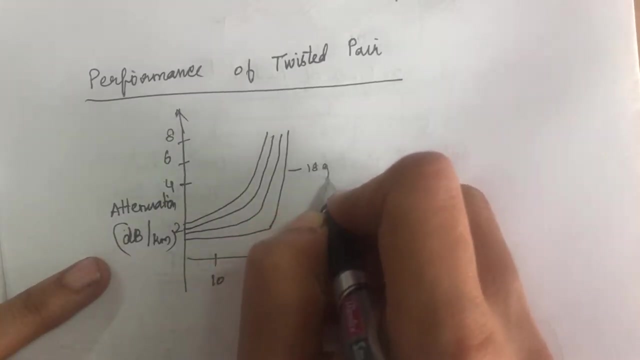 so here this is what the the curve we will get. so here this is what the the curve we will get when it is passed through the transmission medium. so here we are going to compare with for two, four cables: one is 18 gauge cable, other one is 22 gauge cable and the third 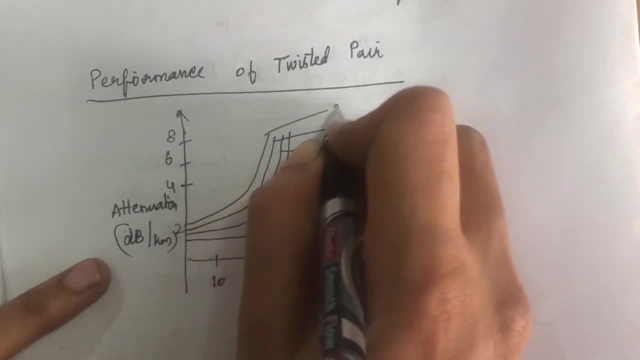 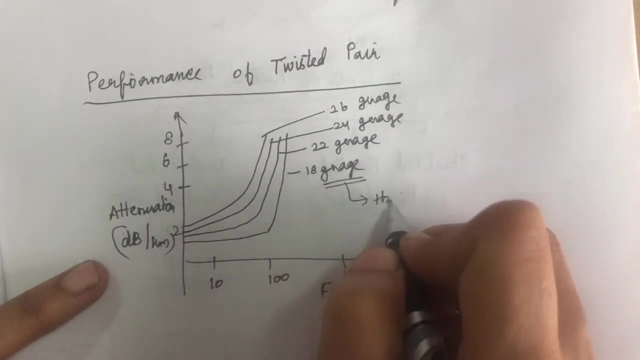 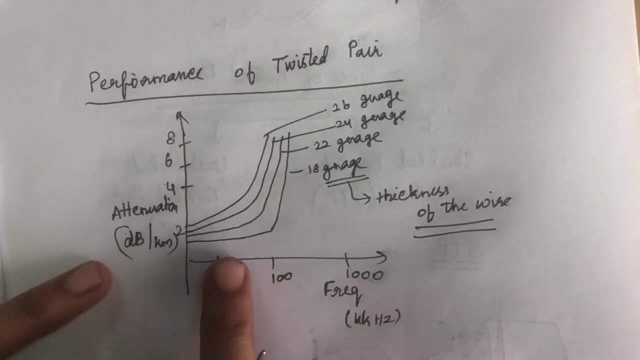 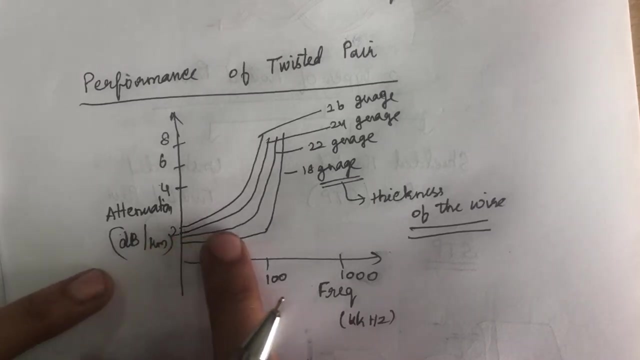 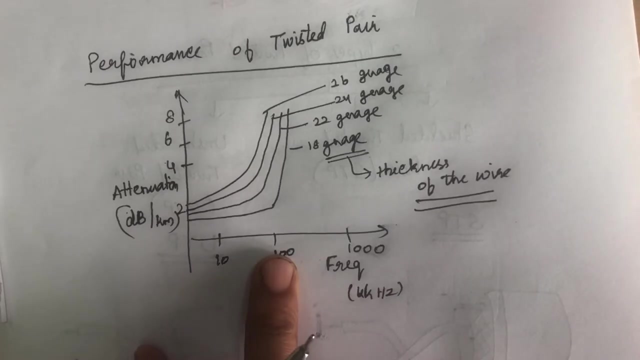 one is 24 gauge and the last one is 26 gauge cable. so here the gauge is nothing but it is the thickness of the wire. so this is what the performance we will get. so here at 100 kilohertz, this attenuation, it sharply increases, it sharply increases above 100 kilohertz. so this is what the performance of twisted pair. 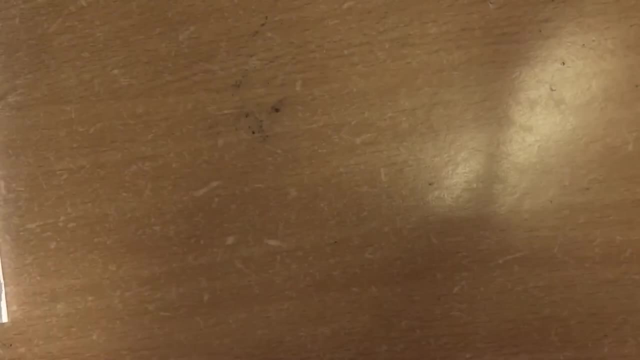 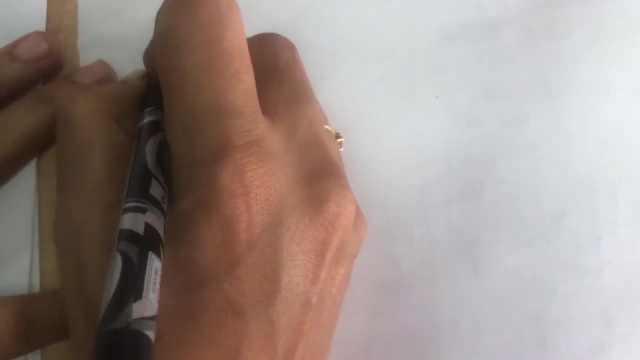 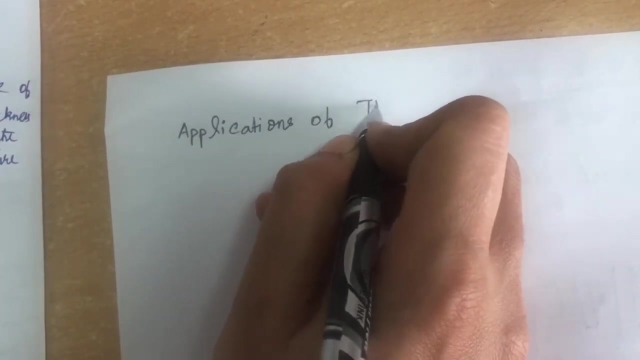 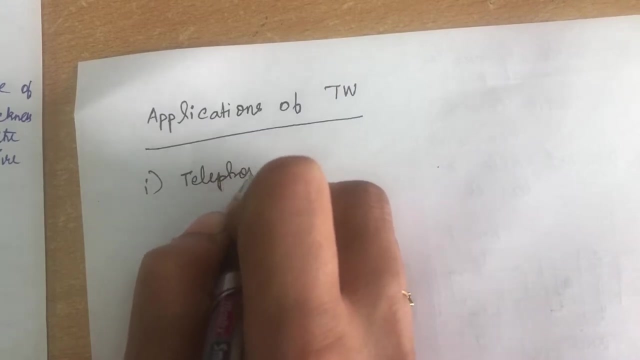 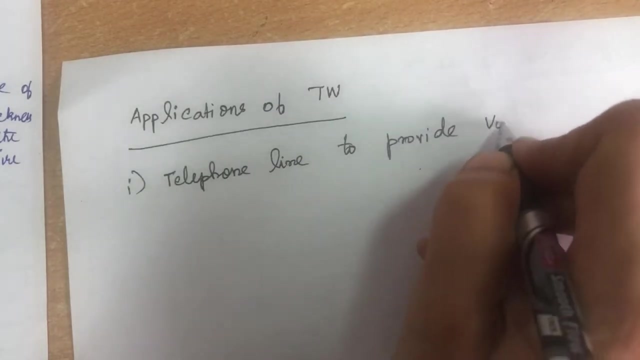 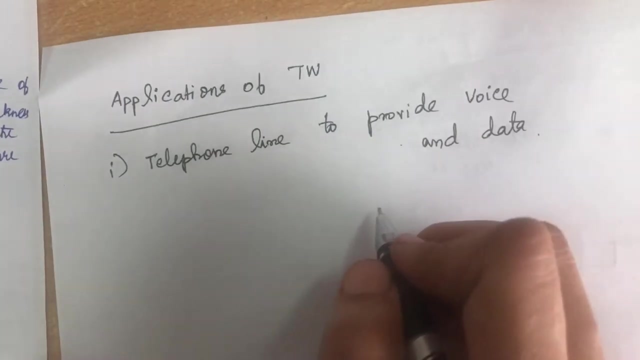 cable. now we will see the applications of twisted pair cable. come to the applications of twisted pair cable. So first application is it is used in telephone lines to provide both voice and data. so in some cases, for example, if you are going to connect the subscribers with the main central, 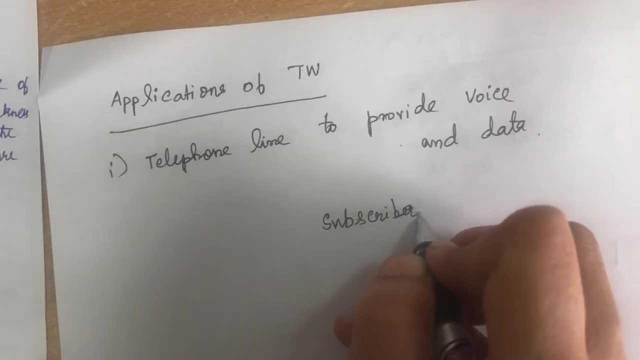 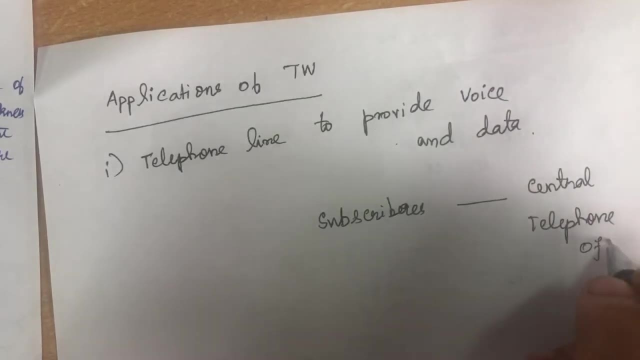 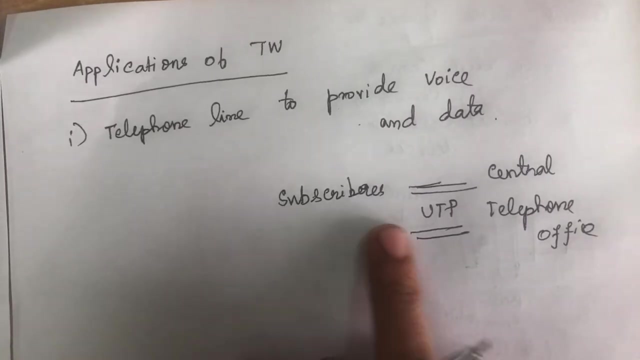 telephone office, so subscribers with central telephone office. in that case, what we can do is we can use an UTP twisted pair- unshielded twisted pair- for connecting the subscribers with central telephone office. okay, these are all the applications. these are all the. 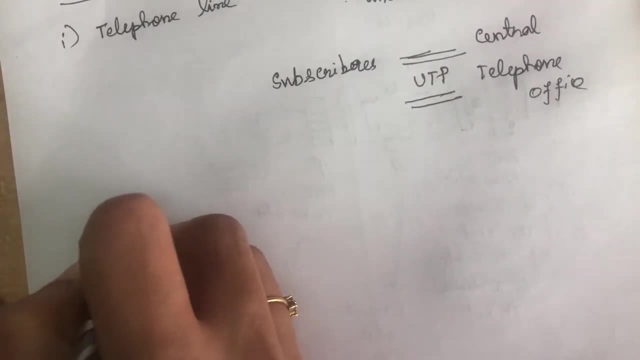 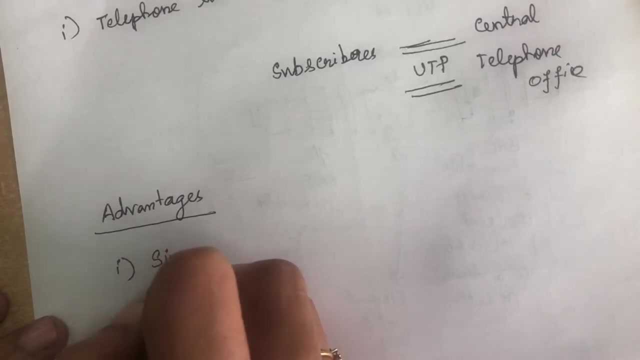 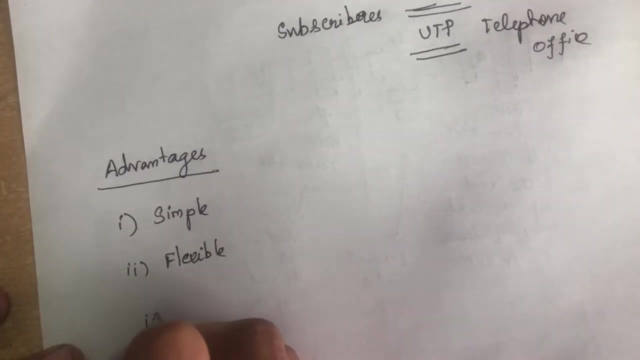 applications of twisted pair cable. Okay, Now we will see the advantages. so, coming to the advantages, it is very simple, okay. the second one is it is flexible, and third is it is easy to install, and fourth is it is cheaper- okay. and fifth one is it is low weight. 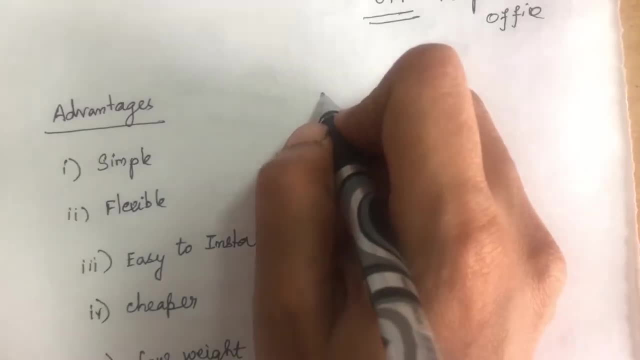 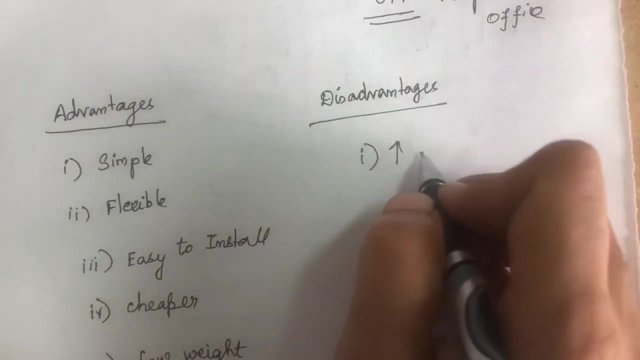 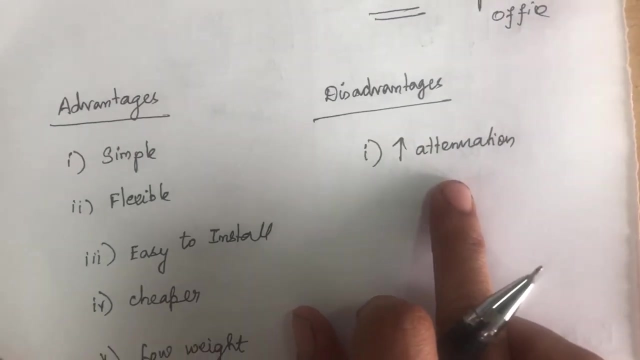 So these are the advantages. So these are all the advantages of twisted pair cable. Coming to the disadvantages. disadvantages: it is having high attenuation, so there will be the loss of the signal will be more when we are going to use twisted pair cable. 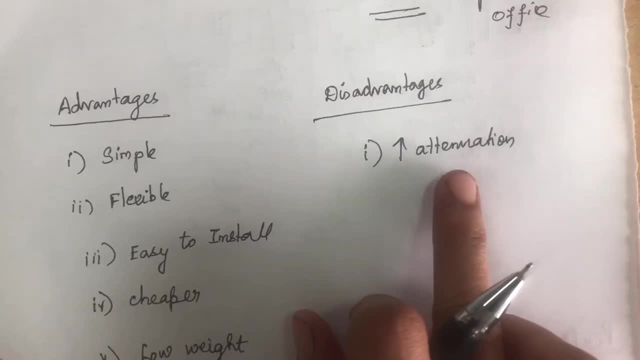 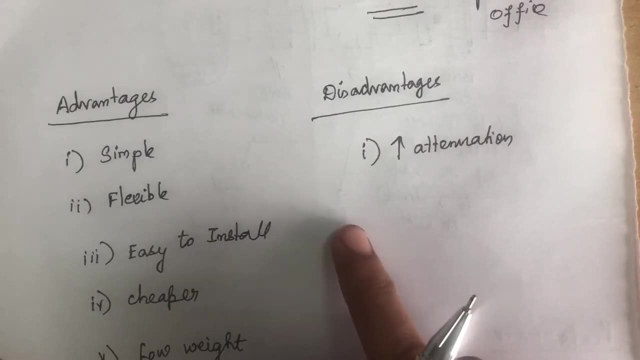 So in this we have seen on twisted pair cable. so here we have. in the twisted pair cable there will be an insulated two copper wires. it will be arranged in spiral pattern. it is of two types. One is unshielded, One is unshielded twisted pair cable. other one is shielded twisted pair cable. 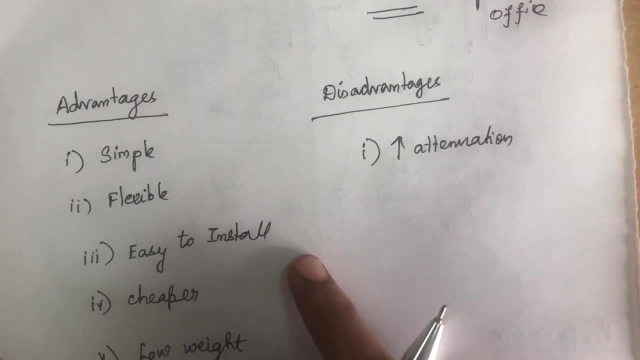 In case of shielded twisted pair cable, there will be a braided mesh which is covering the two copper wires and in case of unshielded twisted pair, there will not be any cover will be there. Coming to this performance of the network, we have seen the performance comparing the 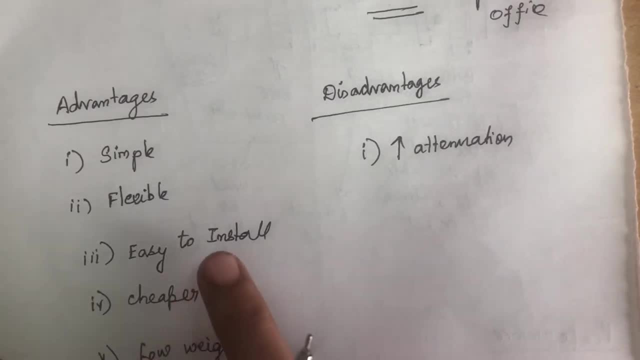 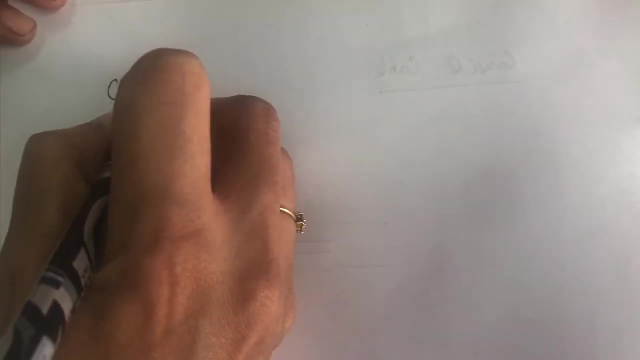 frequency and the attenuation, and we have seen the graph and application. it can be used in telephone line to provide voice and data. and these are the advantages and disadvantages of your twisted pair cable. Okay, Now we will see the next topic in this guided media, that is, coaxial cable. 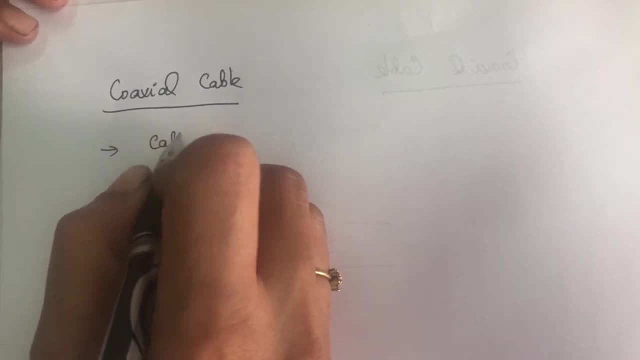 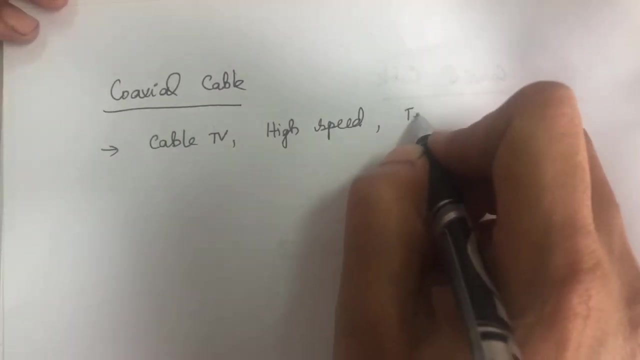 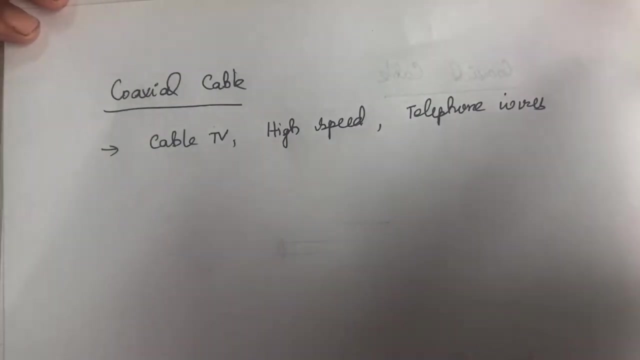 So coaxial cable: it is mainly used in cable TV, or it is used in high speed LAN, or it is used in telephone wires. Okay, So here there will be an inner conductor. Okay, So here there will be an inner conductor. coaxial cable: there will be an inner conductor. 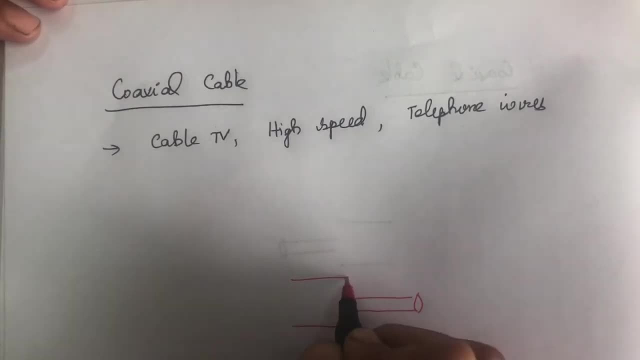 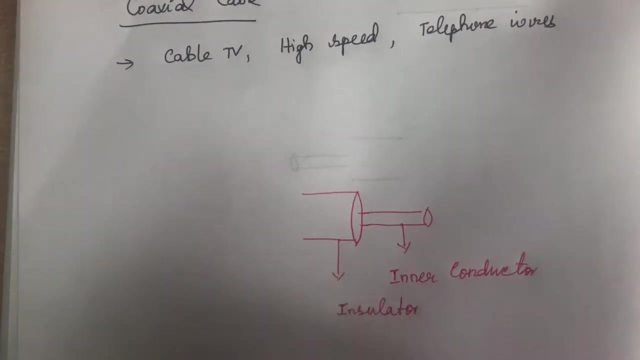 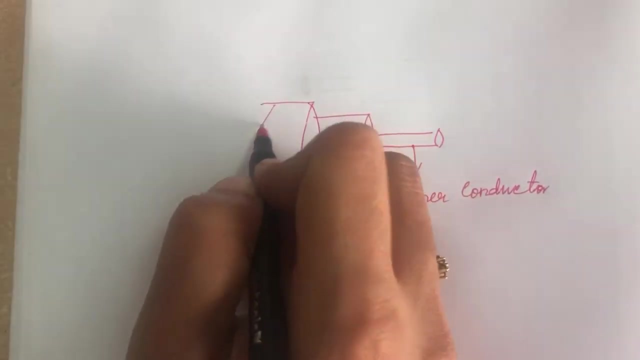 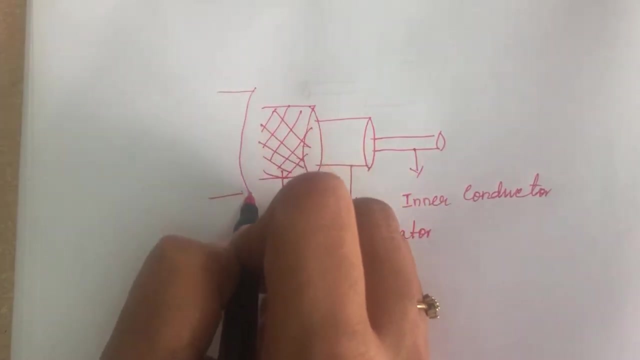 which is surrounded by an insulator like this: This is an inner conductor which is surrounded by an insulator which is again enclosed by an outer conductor. Okay, This is an outer conductor. This is in the mesh format, braided mesh format- and again it is enclosed by an insulator which 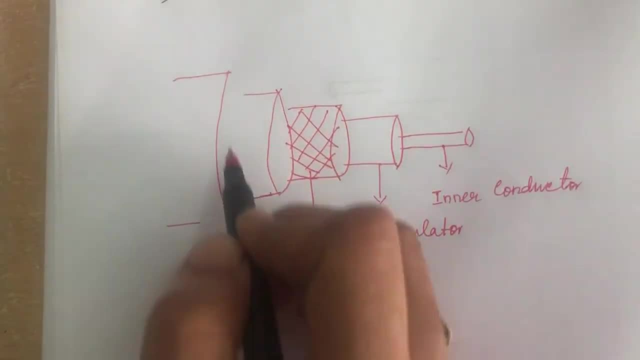 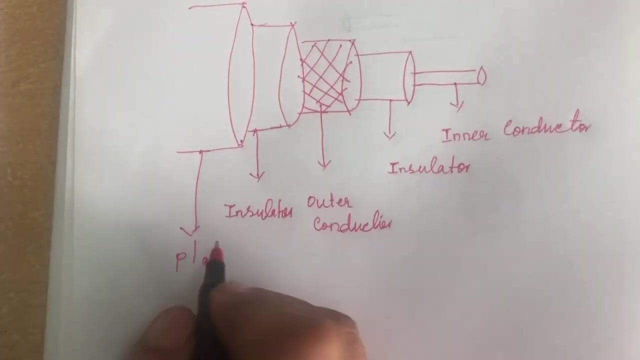 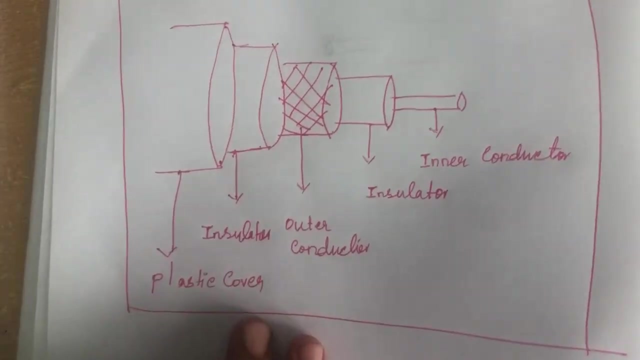 in turn, it is covered by a plastic cover. Okay, So this is the outer conductor. This is the inner conductor. Okay, So this is the structure of the coaxial cable. So the coaxial cable will have an inner conductor, which is, in turn, surrounded by an insulator. 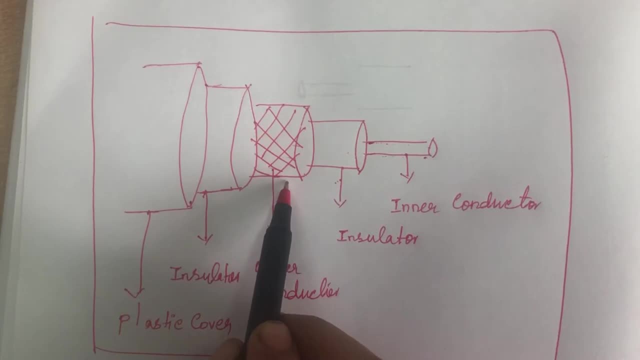 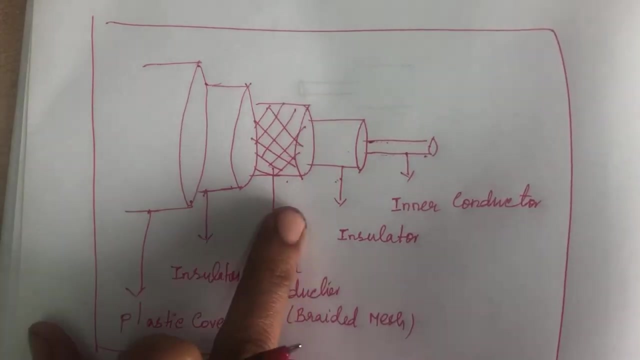 or inner insulator, and again it is enclosed by an outer conductor which is braided mesh, which in turn it is enclosed by an outer insulator which is again covered by a plastic cover. So this is the structure of the coaxial cable. Okay, 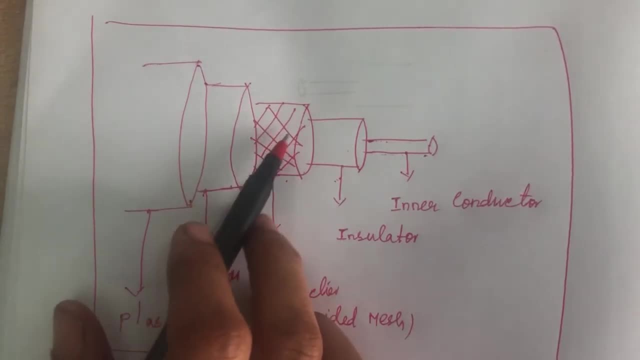 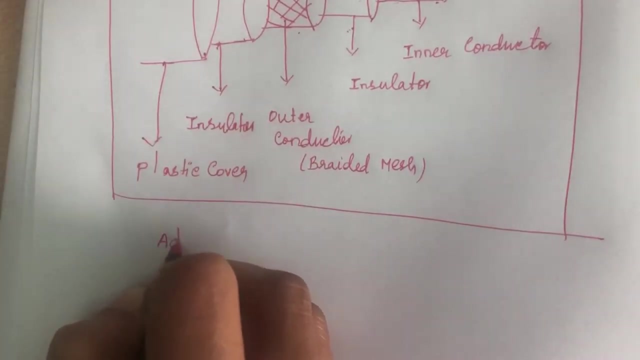 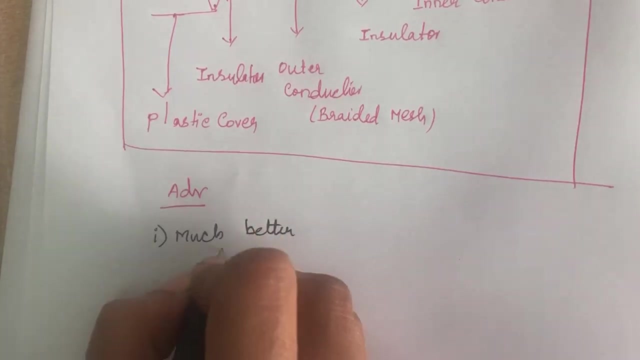 So this shield, this metallic wrapping, or this braided mesh, will protect from noise and as well as other interferences. Okay, So this is the structure of the coaxial cable. So this coaxial cable coming to the advantages of coaxial cable, it is much better since saturation. 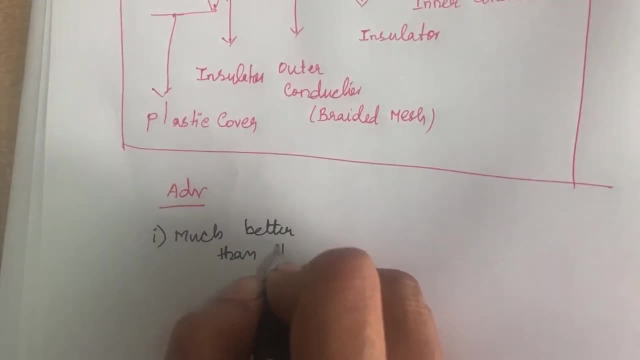 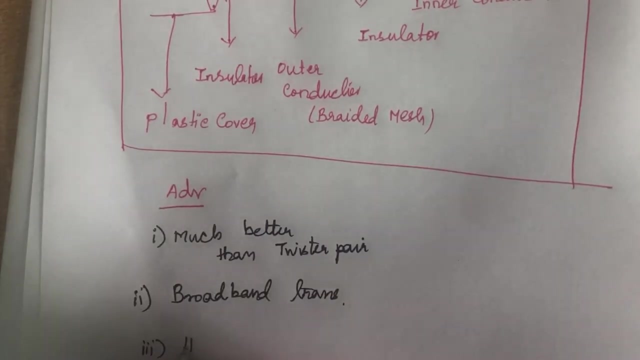 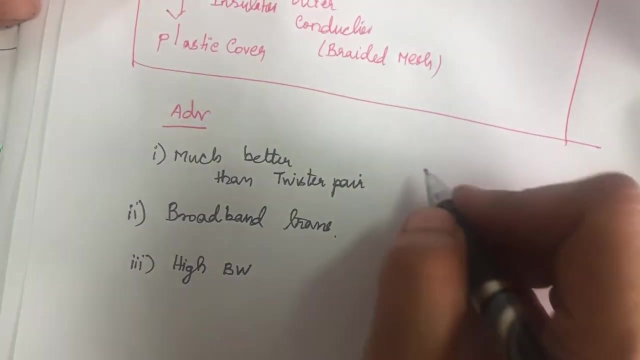 is less compared to twisted pair cable. it is much better than twisted pair. Okay, The second is it is used for broadband transmission and it works for higher bandwidth too. it works for higher bandwidth also. coming to the disadvantages, one is it is expensive in compared with the 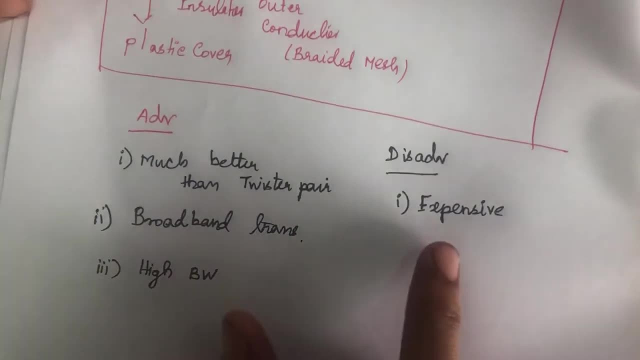 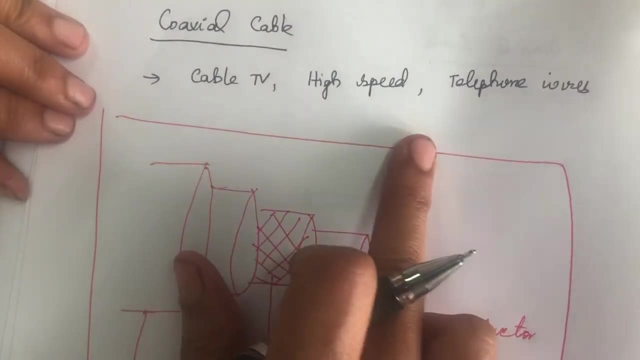 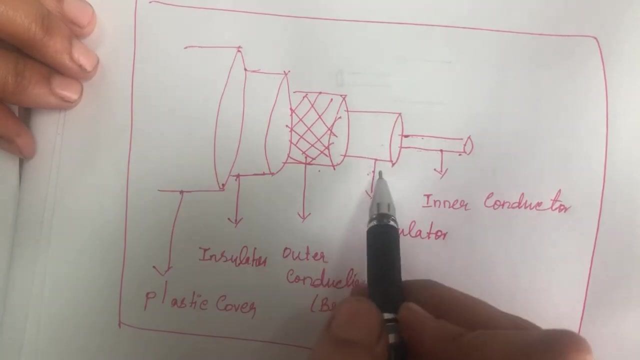 coaxial cable. Okay, When compared with twisted pair, it is very expensive. So here this coaxial cable. it is mainly used in cable TV, high speed or telephone wires, and it is having an inner conductor which, in turn, it is surrounded by an insulator which 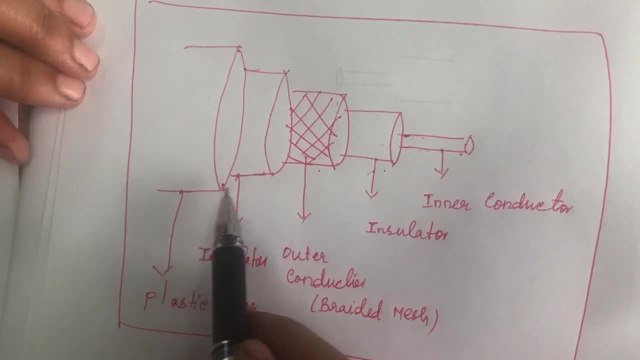 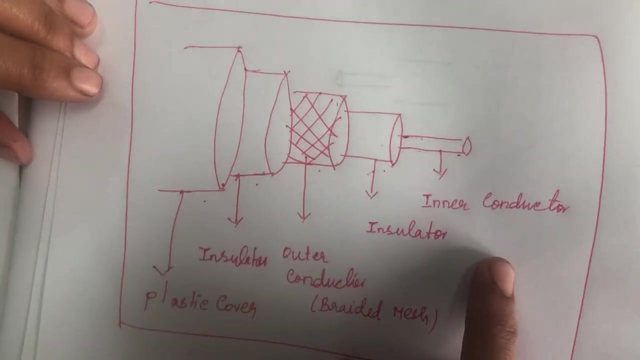 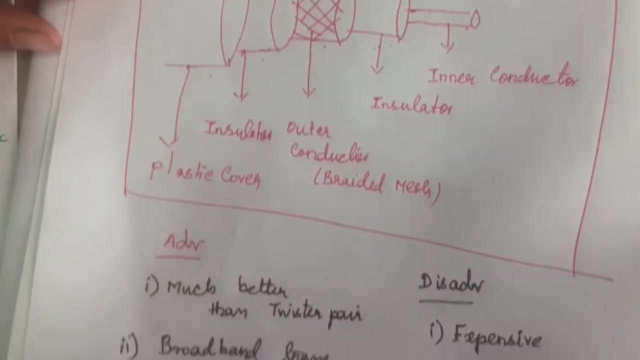 in turn. it is enclosed by an outer conductor which is covered by insulator and plastic cover. So the wire, the signals it is transmitted through this particular transmission medium will be very safe and it is very secure. That is why, in most high speed transmission you will be using this type of coaxial cable. 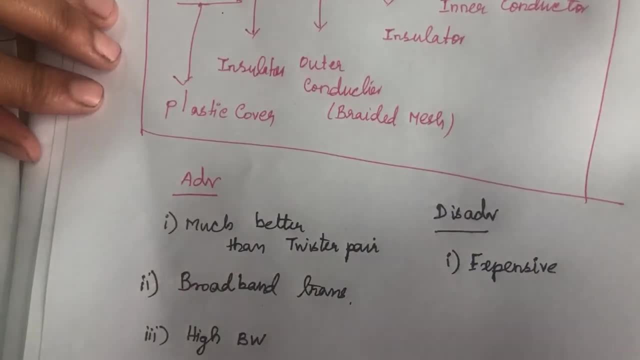 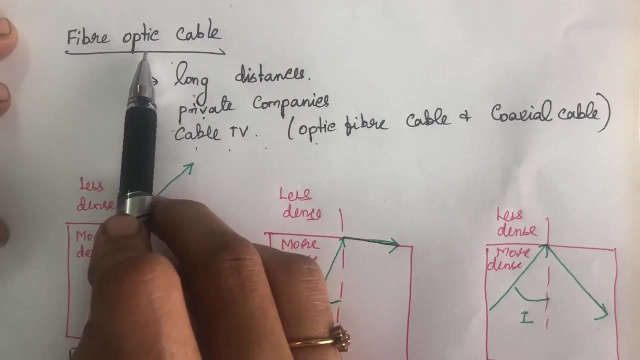 and these are the advantages and disadvantages of coaxial cable. Now we will see the last cable in guided media, that is, fiber optic cable. So fiber optic cable, it is used for communicating in longer distances and it is used in private companies where high speed communication is required, and it is also used in cable TV communication. 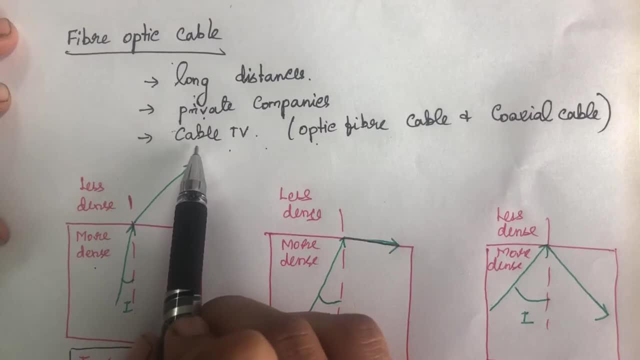 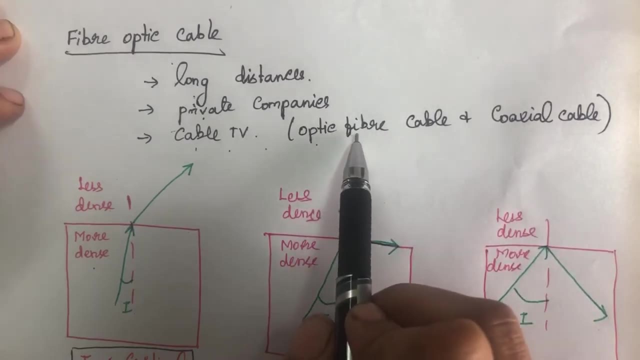 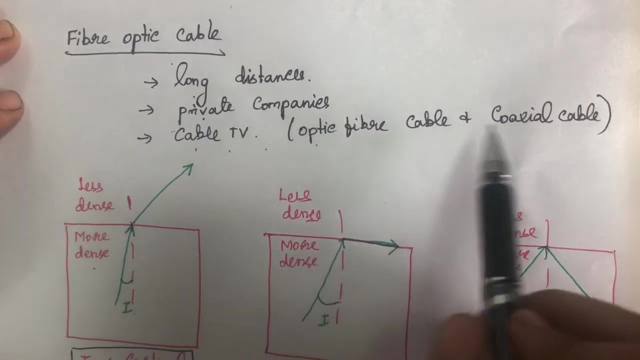 But they will be using both the type of network- optical fiber cable and as well as coaxial cable for communication. So these type of combination of networks is called as hybrid network, where optical fibers will be used in the act as a backbone for the network and coaxial cable will be connected. 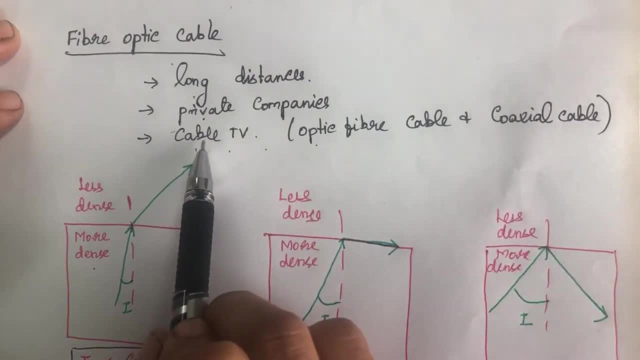 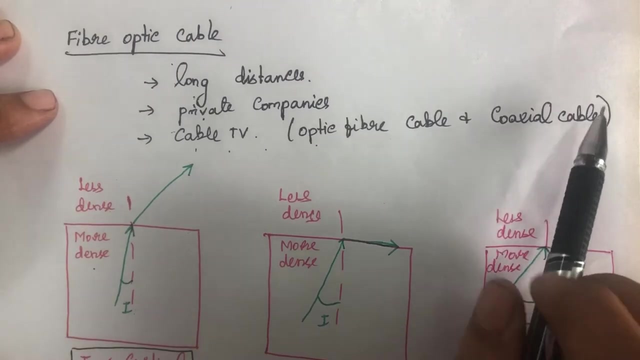 to all the user premises. So this cable TV, when they are going to use a combination of these two types of cables, then they will get the user, it will be cost effective and also they will get high bandwidth. that is why they are using a combination of these two. 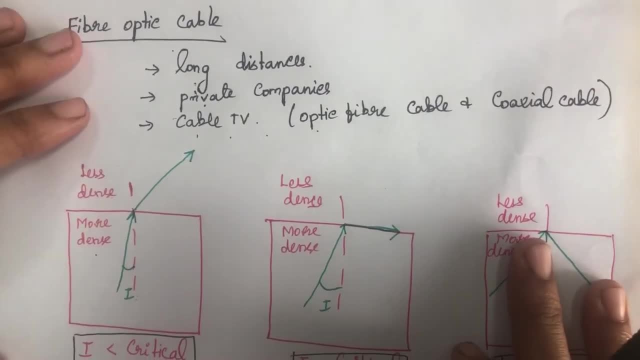 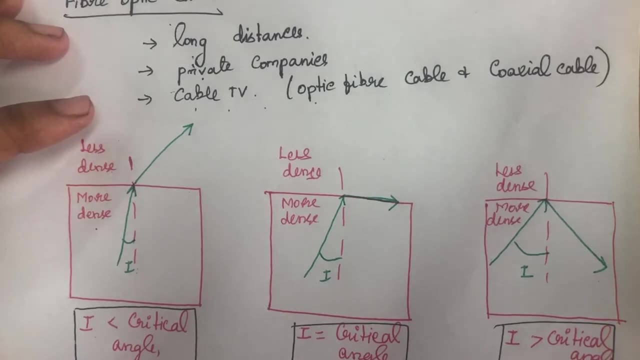 So now we will, before going in detail about fiber optic, we will see the aspects of light. when a light travels in the same medium, that is, in the same medium, it always travels in the straight line. When a light travels from one medium to another medium, there will be the ray of light will. 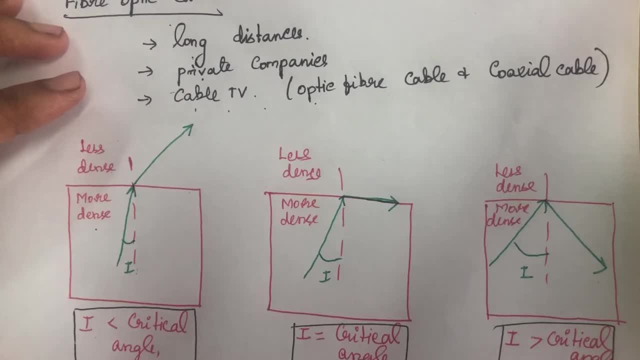 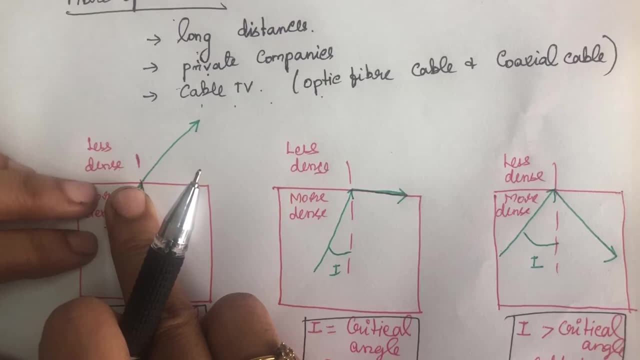 gets reflected or refracted based on the density of the medium. So here we are going to see how the light, ray of light, it gets reflected or refracted because of change in the density of the medium. So here when the ray of light, when it stands for, when it passes from the more density medium. 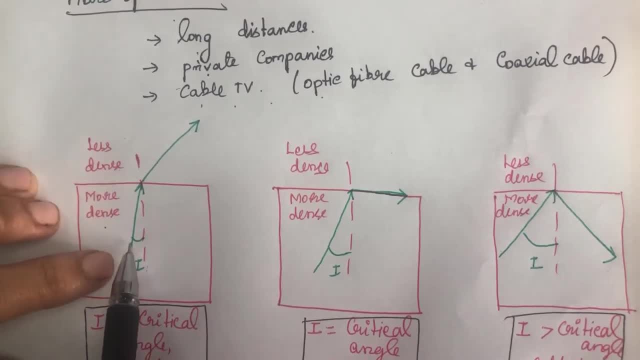 to the less density medium. So what happens is that that the ray of light is lesser than the critical angle. the ray of light will get refracted, and refracted from the interface. So here in this second diagram. so here what happens is that when 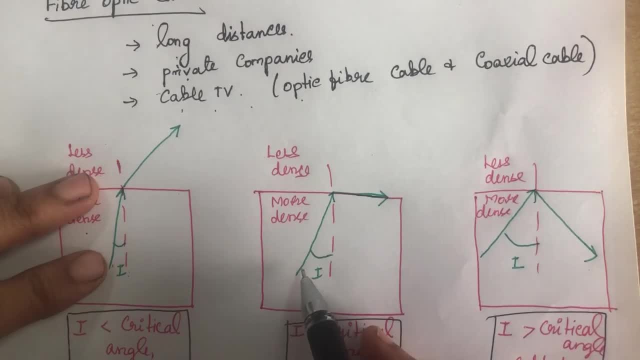 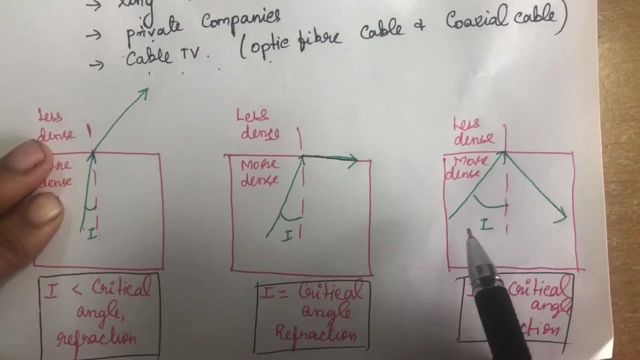 the ray of light if it is equal to the critical angle. so ray of light will, instead of going refraction, it will coincide with the surface of the medium interface. that is more, it will be in the. it will be coinciding with the medium and the third diagram. so here, when the ray of light 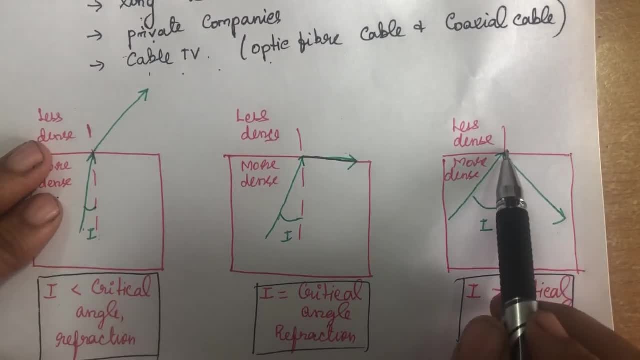 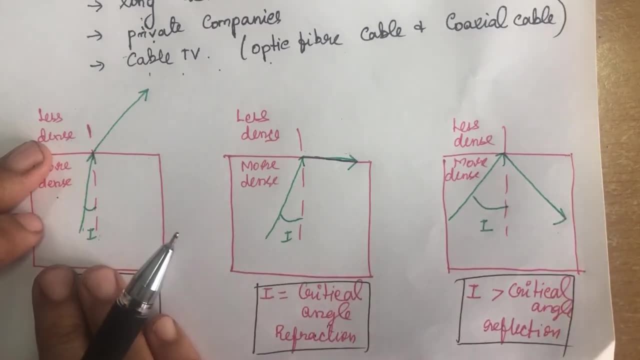 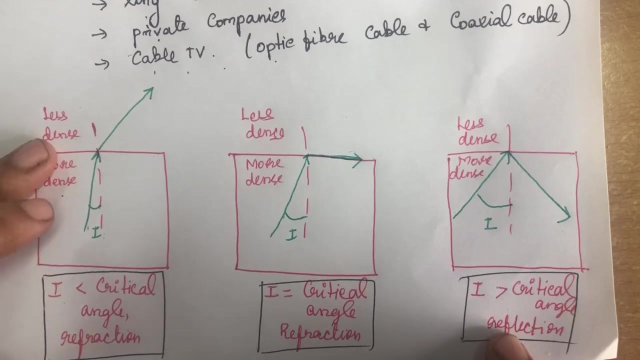 if it is greater than the critical angle, instead of getting reflected refracted, it gets reflected inside the medium. So here, optical fiber, it chooses this third property, that is, it gets when, it, when, the when, when it is traveled through a medium high, more density medium to less density medium. 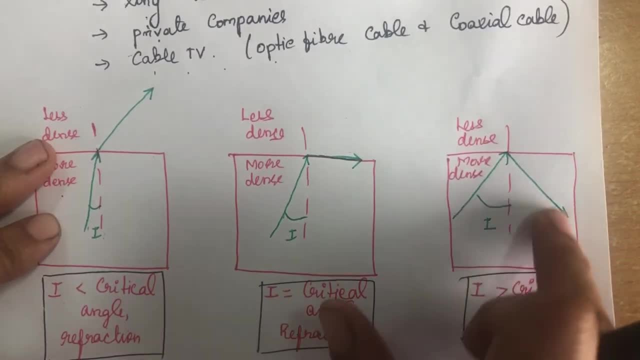 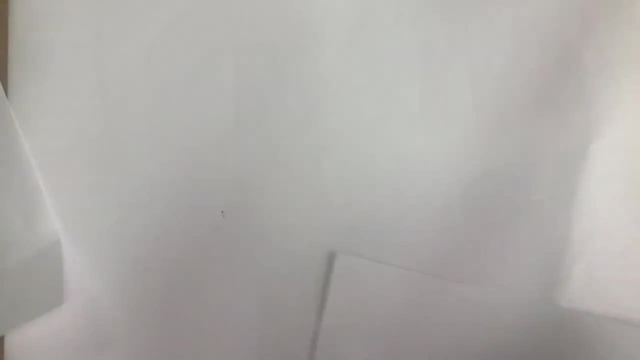 if this ray of light will get reflected, and it will get reflected inside the medium. So here, optical fiber, it chooses this third property, that it will comes inside the medium itself. So now we will see how optical fiber, the structure of optical fibers. So, coming to the structure of optical fiber, it is made up of a, it is having 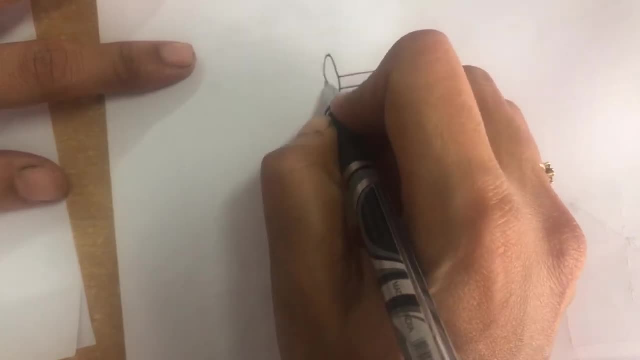 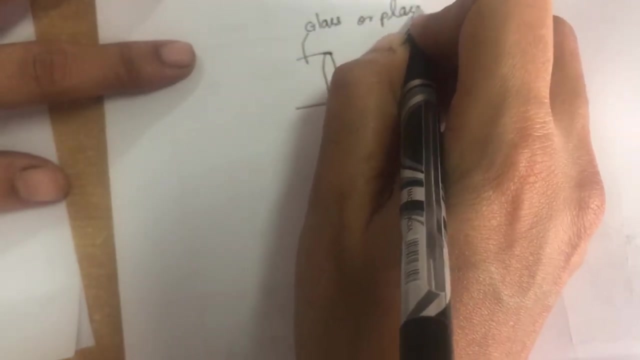 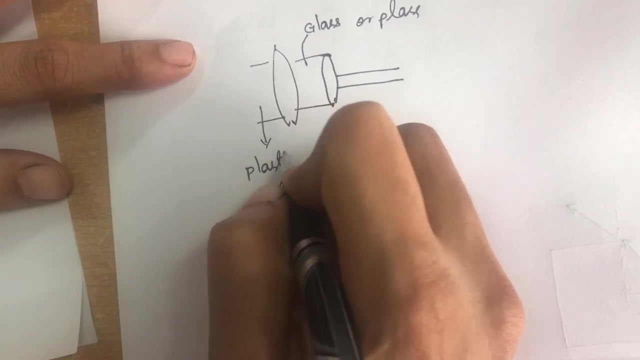 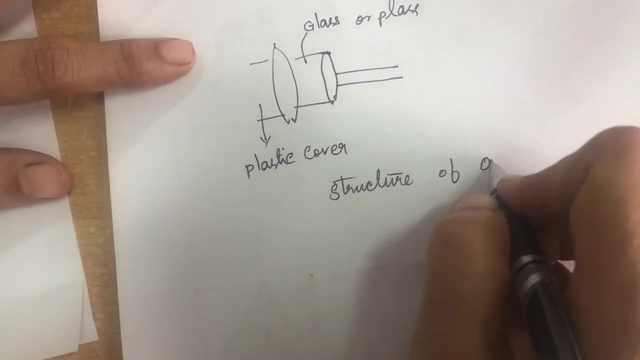 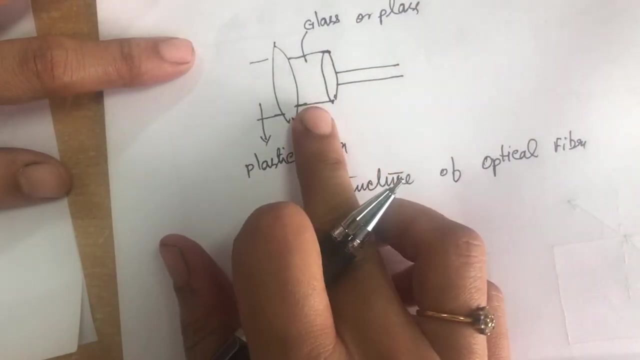 a core, this cable, it will be connected, it will be enclosed with a glass or plastic, a. So again this, James, glass or plastic is enclosed with plastic cover. so this is a structure of brush optical fiber. So a copper wire will be enclosed with glass or plastic. and again, which is again, 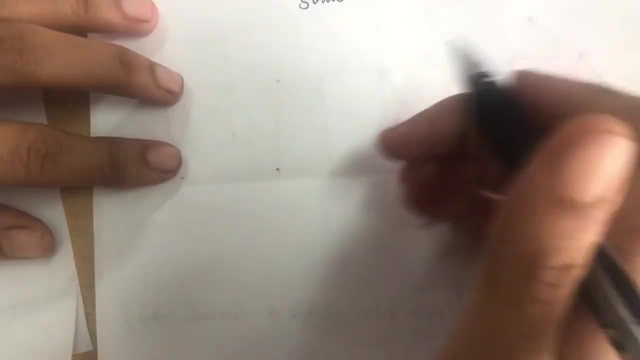 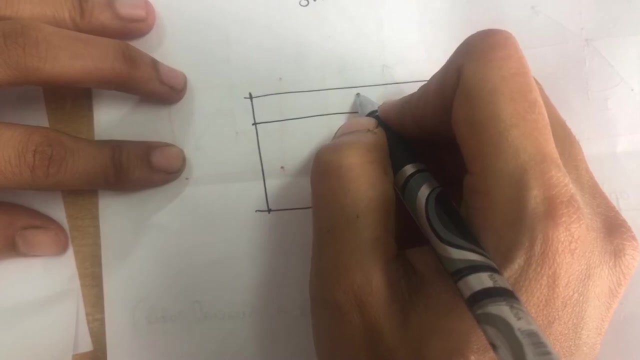 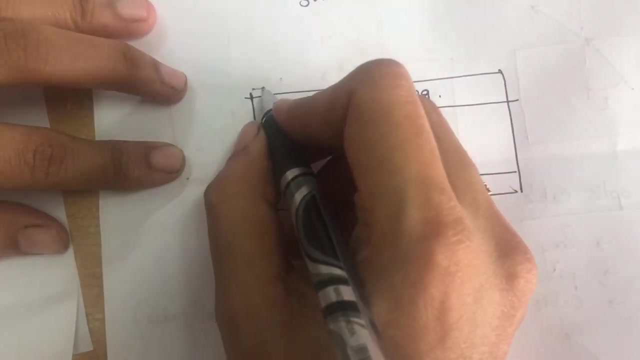 enclosed with plastic cover. so this is the, the structure of optical fiber, so anything can be. Pierce Мыeleri�� flexible cityıyoruz, So we can also draw like this. so this is the- we can call this glass or plastic to be cladding, and there will be an outer cover over here. 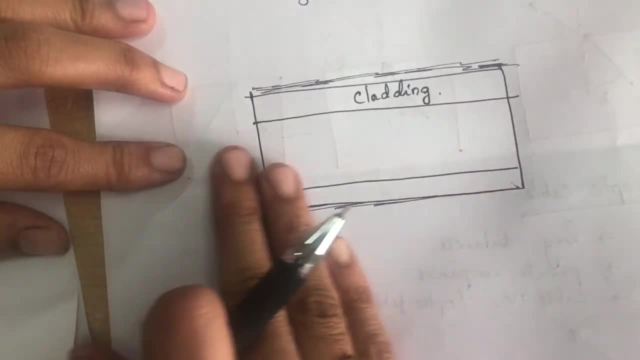 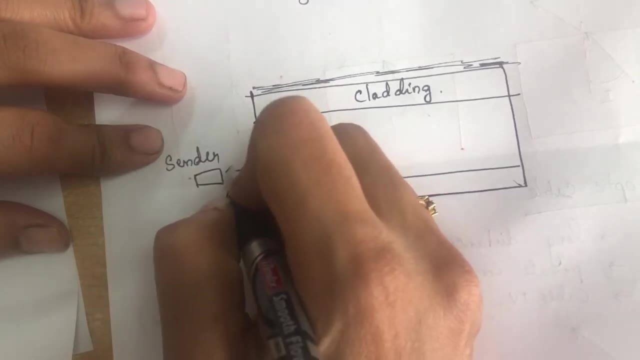 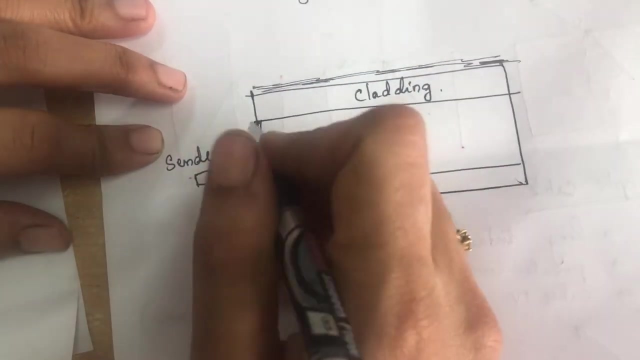 So inside this there is a conductor, here the signals will be passed. suppose, for example, the sender is sending a message. so when it has been sent, since it is, this glass or medium is different medium and here it is having a different medium. so what happens is that 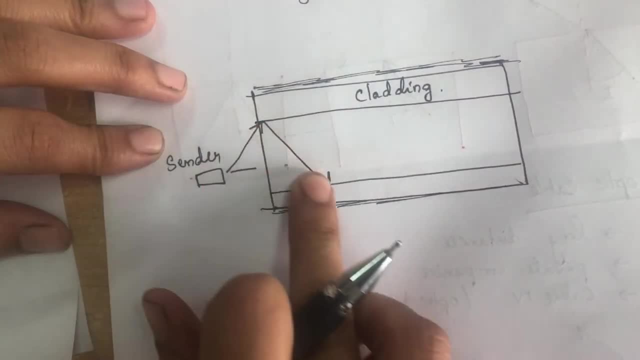 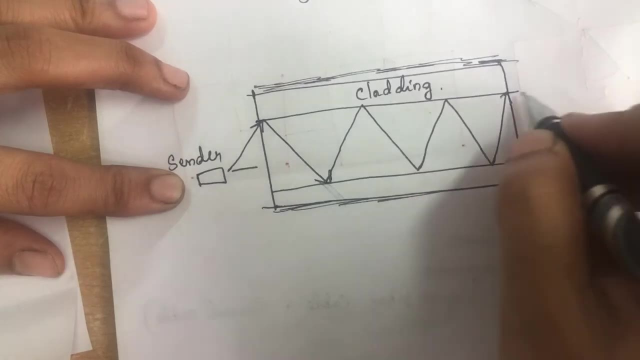 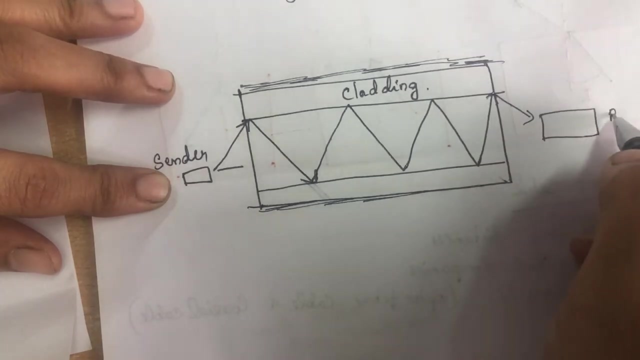 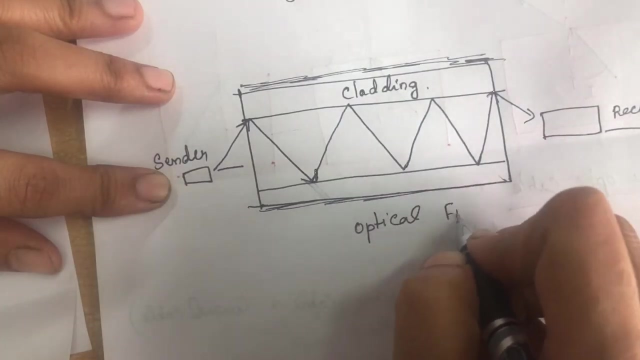 it gets reflected and it goes. the ray of light will goes inside this and again, it gets reflected inside the core and, at last, it reaches the end of this cladding. it comes outside and thus the receiver will receive it. The receiver will receive the message. 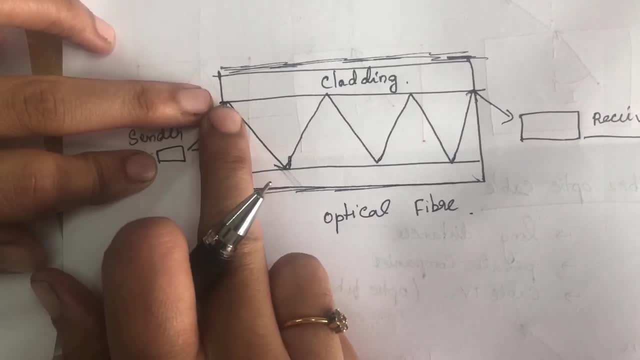 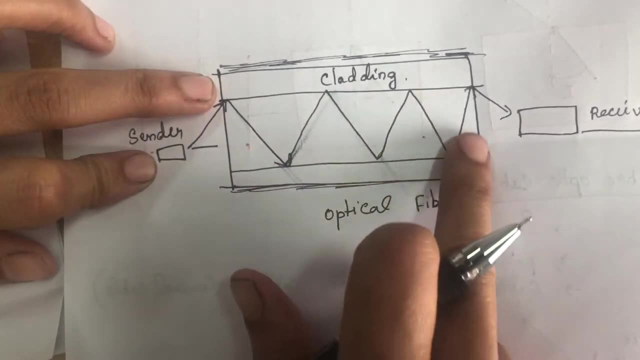 So here, when the sender sends a message, so here the ray of light. since it is passing from more density to lesser density medium, it gets reflected, again back it gets reflected and at last it reaches the end of the wire. now the receiver will receive the message. 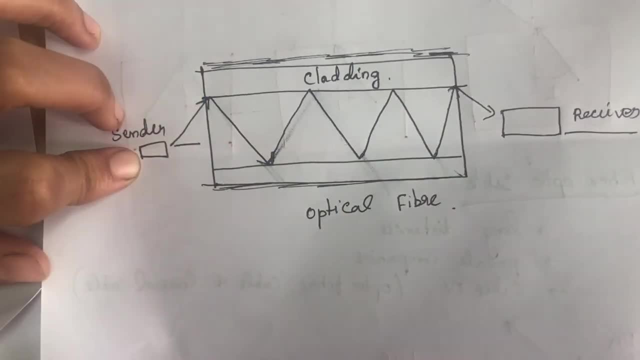 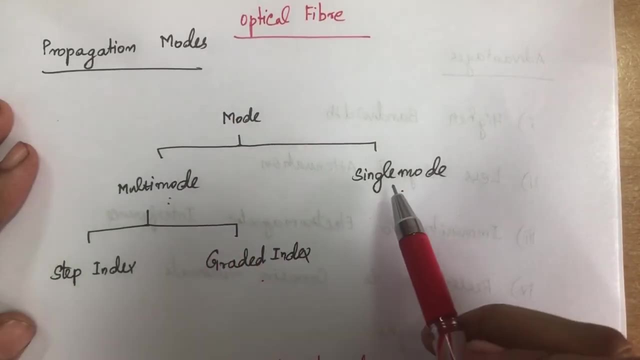 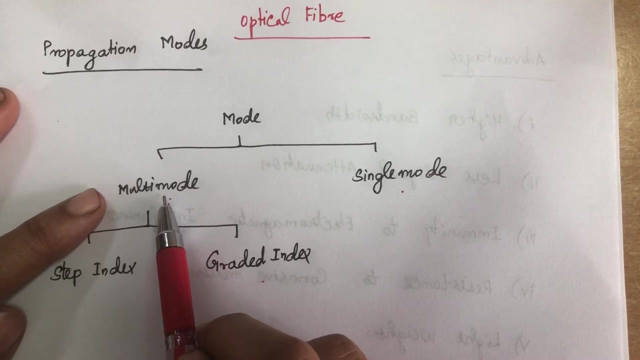 This is how the optical fiber will send the message inside the medium. Now we will see the propagation modes of optical fiber. So propagation modes are divided into multi mode and single mode. and again this multi mode is divided into step index and graded index. So what is multi mode? transmission is here. this optical channel will allow multiple beams. 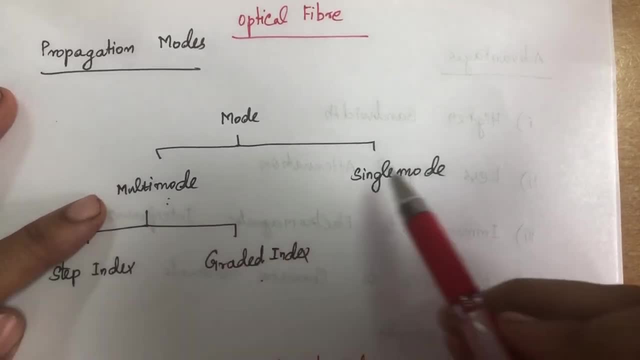 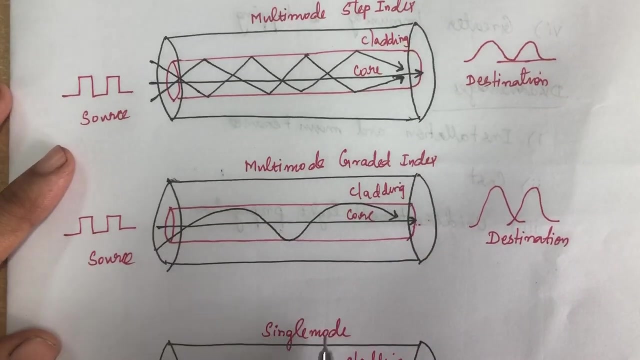 of light to pass through the channel. that is multi mode. and single mode is it will allow only one beam of light to pass through the medium. that is single mode. So we will see The diagrams for multi mode, step index, multi mode graded index and last is single mode. 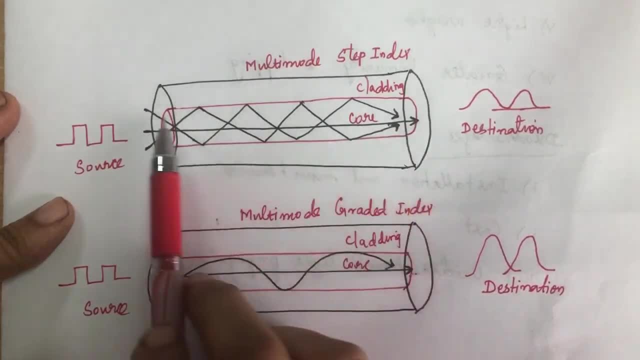 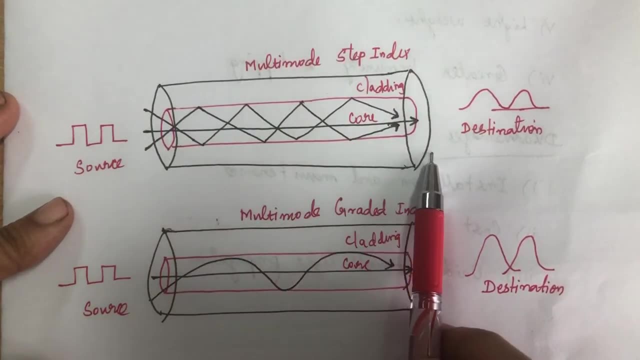 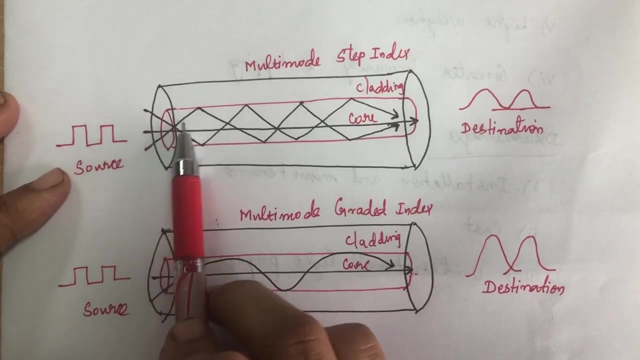 Coming to multi mode step index. this is the core of the transmission medium, and outside we have a cladding and outside we have the plastic cover. So here, when the source sends the message inside this transmission medium, several beams of light will be passed inside this medium. 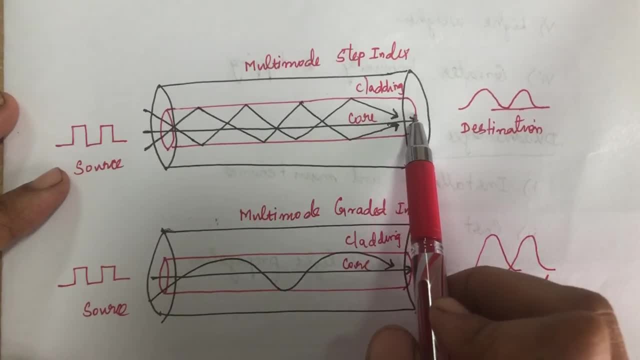 It gets reflected And it reaches the edge of this core. Here the density of this core will be constant from the center to the edges. So once if it reaches the edges here it has to move to the next outside cable where it is having lesser medium. 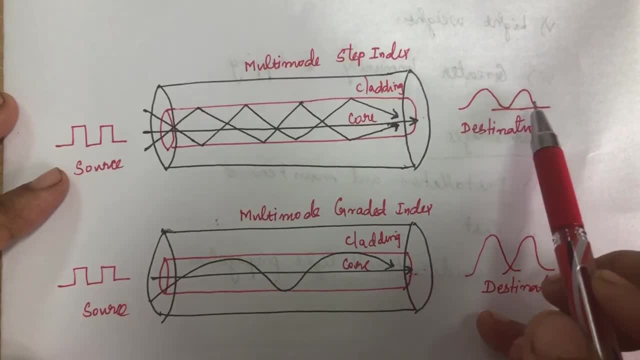 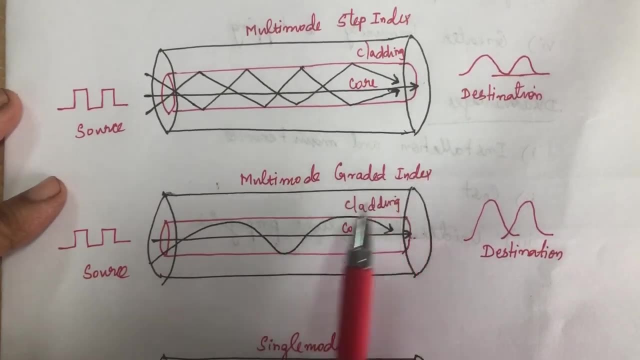 So here what happens is the distortion occurs only at the edges. This is what the output we will get at the destination. Now coming to multi mode graded index method. Here also, The source will send the message. here, multiple beams will travel through the this density. 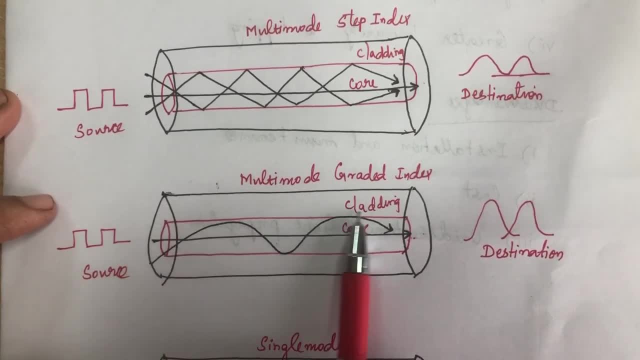 through this core. Here what happens is that the density of the core will be highest at the center and it will be lower at the edges of this core. So once this ray of light it passes, it goes to the edges of the core. outside medium is: 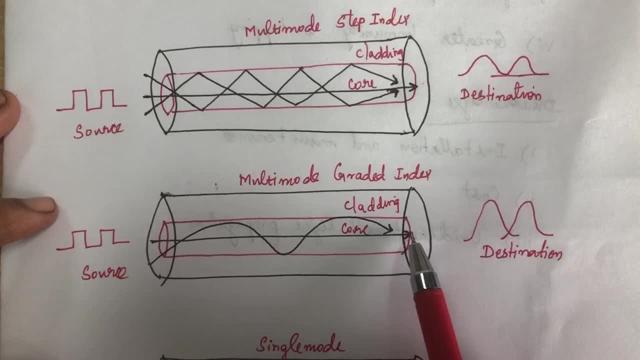 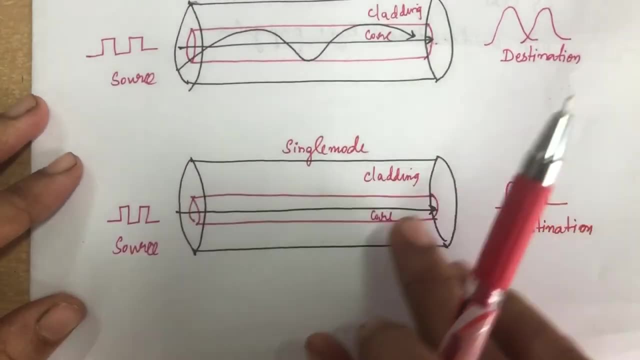 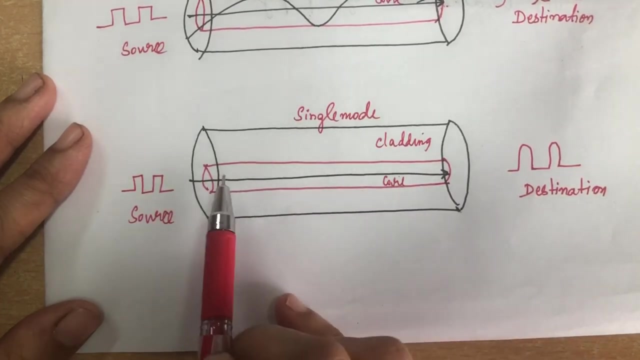 also lower, and here also it is having a lesser medium. So what happens is distortion will be less at the edges. This is what we have got The receiver. now we move on to the single mode transmission. in single mode, only one beam of light will be passed inside the core. 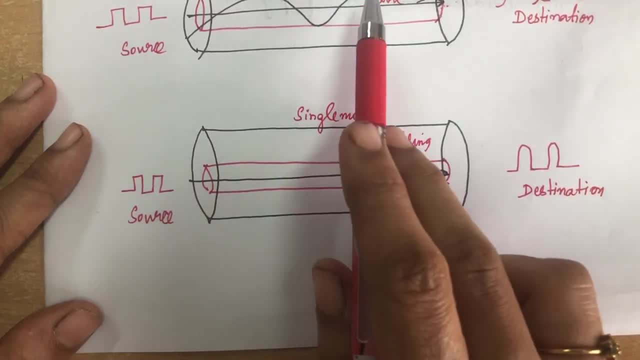 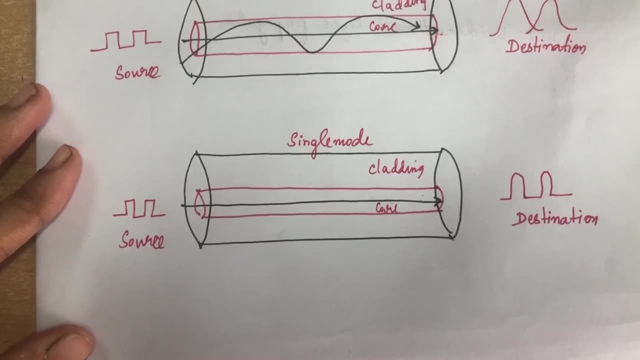 So the radius of the core will be less when compared to other two methods. So it passes and reaches the end and this is what the output we will get at the destination. So in this topic we have seen several propagation modes- multi modes, single mode- and we have seen in detail about step index and graded index with the single mode need diagram. Now we will see the advantages of optical fiber. The first advantage is higher bandwidth. So this fiber optic cable support higher bandwidth than the coaxial cable and twisted pair. Second is less signal attenuation. Usually this optical fiber can travel longer. distance. even though it is traveling in longer distance, it will have less attenuation. Suppose if you are going to use fiber optic, other twisted pair or coaxial cable for 50 kilometers. Suppose you have to run a signal inside, run a signal for 50 kilometer. So in that case, for every 5 kilometer.